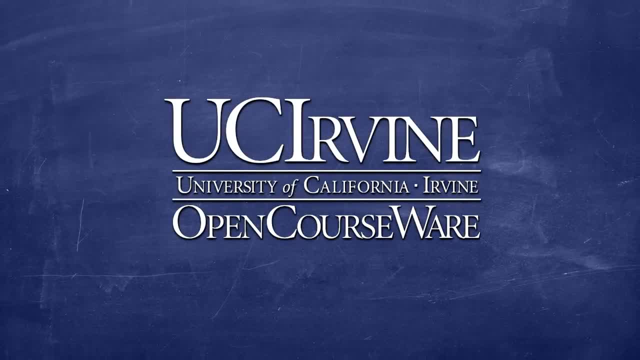 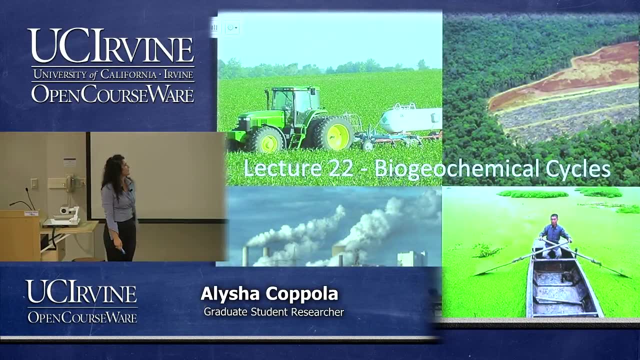 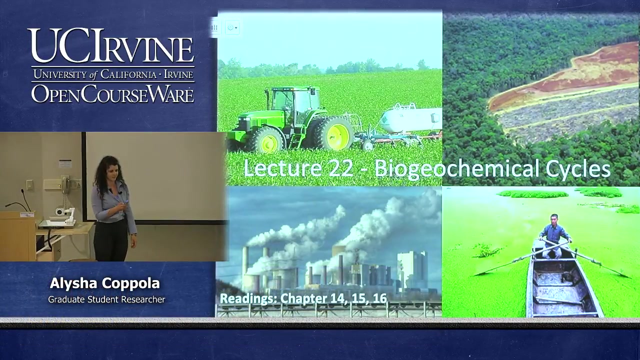 Thanks, Thanks. Okay, So I study biogeochemical cycles, mostly carbon and the ocean. So today we're going to talk about all different biogeochemical cycles and the most important ones and how they operate and how they may have changed with human influence. Okay, So what is a biogeochemical? 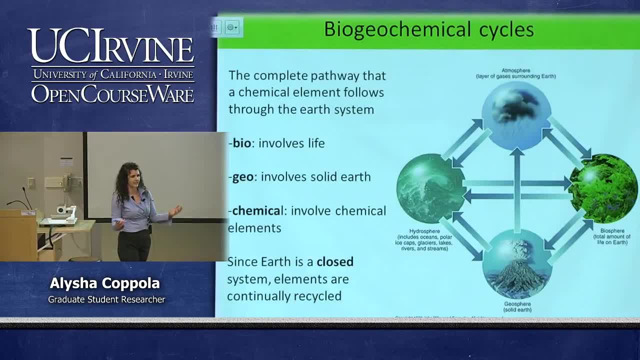 cycle. So bio it involves life, So it's anything involving life. Geo it involves the solid earth, And chemical it involves the chemical transformations through each of these spheres, So through the hydrosphere, through the atmosphere, through the geosphere. And there's different. 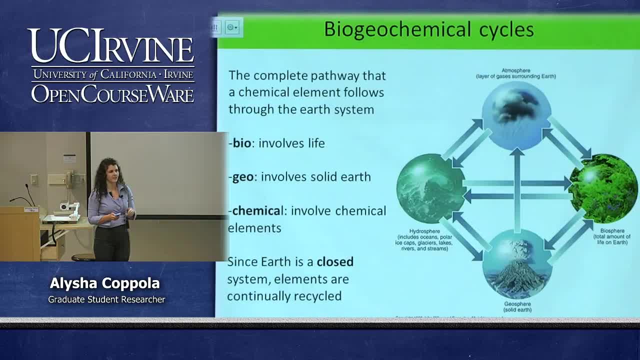 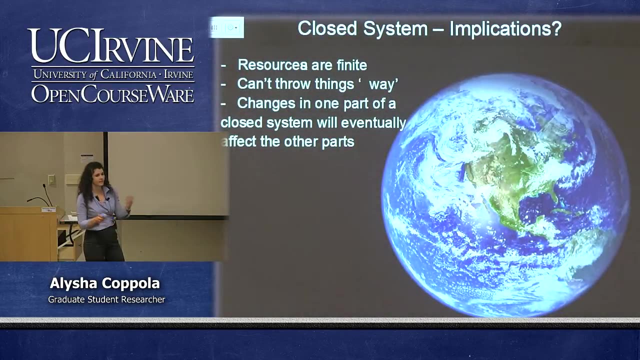 transformations and transfers from each of these spheres And they operate together as a closed system. but the atmosphere, for instance, is operating with exchanging between each of these within the earth system, So together it's a closed system and each of these different. 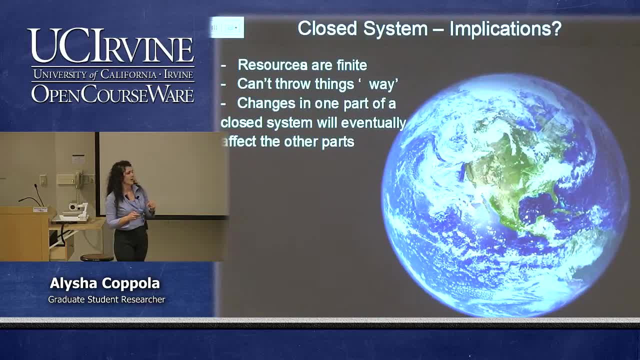 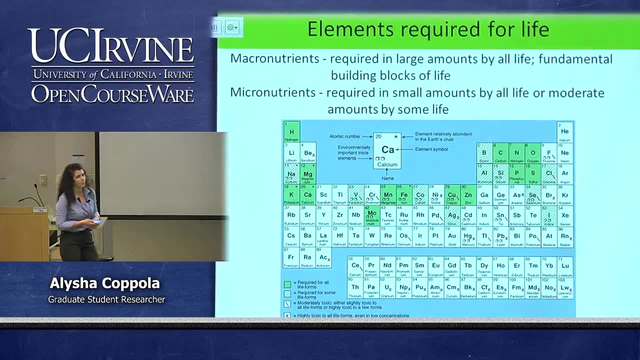 systems are closed together, but we're looking at the transformations between the atmosphere, biosphere, geosphere and hydrosphere. So what elements are required for life? So we divide them up into macronutrients and micronutrients. So macronutrients are required. 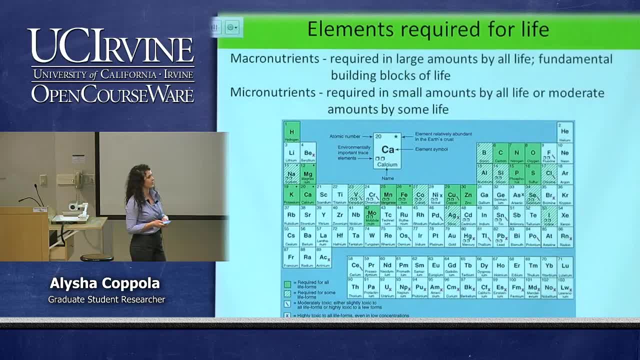 in large quantities and they're essential for life. So, as you can see in green on this periodic table, those are the elements that are required for all of life forms, And micronutrients are required in small amounts, So there may be not high concentrations and they're not. 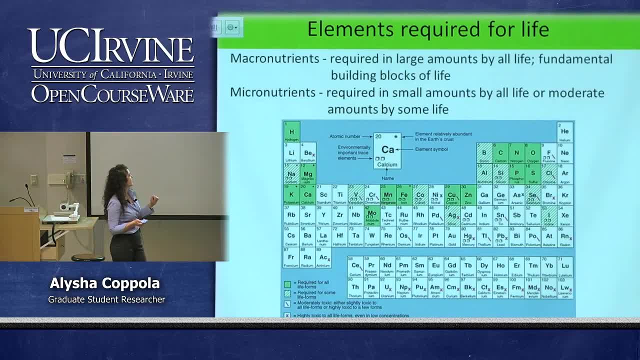 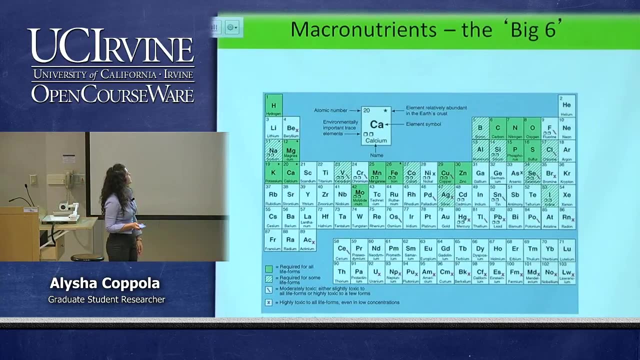 essential for all life forms. So we divide them up into macronutrients and micronutrients. life forms and those are in the dashed green. so that might be like copper that's required in small concentrations but not as important as something like carbon that we all need for growth. so within the macronutrients we're dividing. 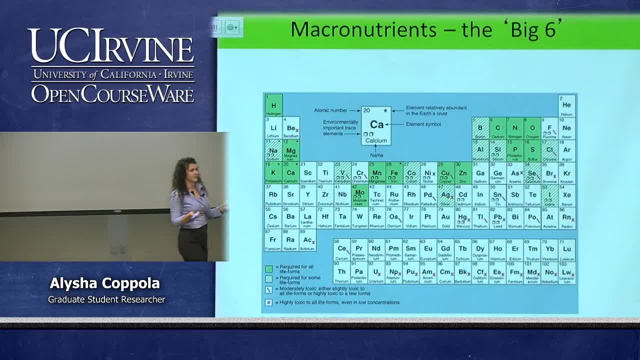 it up into the big six. so, like, what's the biggest, most important elements that are required for life? so does anyone have any ideas of what, within those green shaded elements, which ones are the most important, or which is the most important or one of the big six? yeah, carbon, so we have carbons very important. 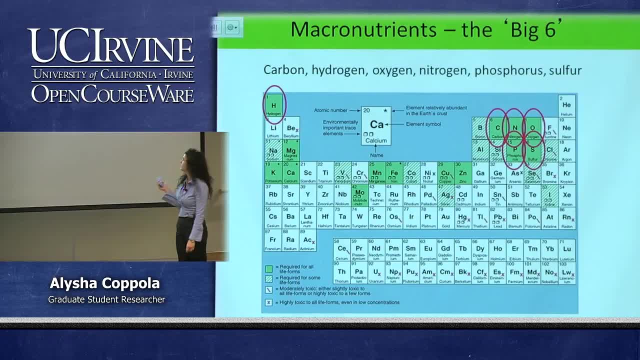 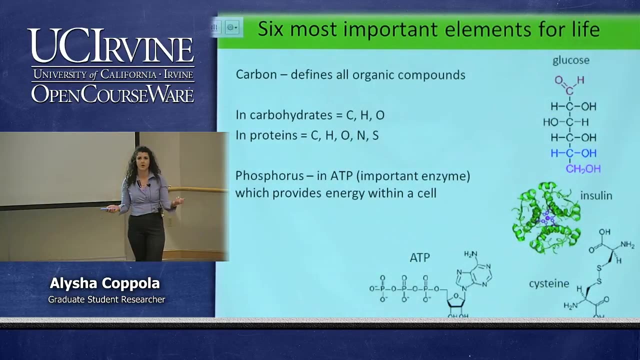 we'll be talking about that today. nitrogen, oxygen, phosphorus, sulfur and hydrogen are the big six, so those are the ones we're mostly concerned about. so go ahead and read the next slide. carbon, as you all know, is most important because it makes up all organic compounds. it's the most important and everything involves carbon. 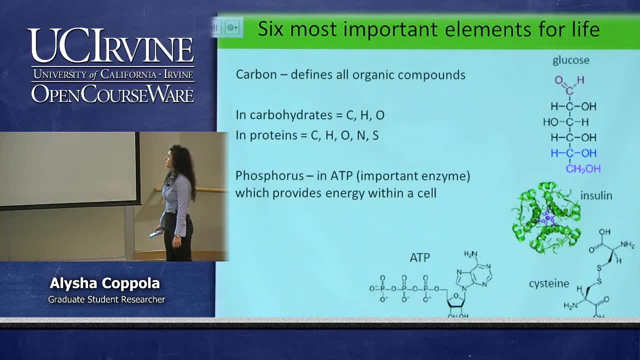 so it's in carbohydrates, it's in proteins and amino acids, and we also have the presence of hydrogen and oxygen, and nitrogen is also in part, important, in that we have phosphorus, which is important in ATP and ADP, which is important for getting energy within the cell. 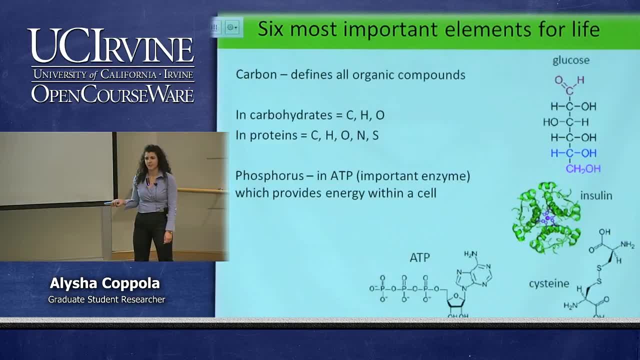 sulfur is important, as Julie talked about previously. at mid-ocean ridges you have these hydrothermal vents and that's a source of sulfur, is a source of energy for those ecosystems deep in the ocean along the North Atlantic Ridge. so these are the most important elements that are required for life on earth. these other 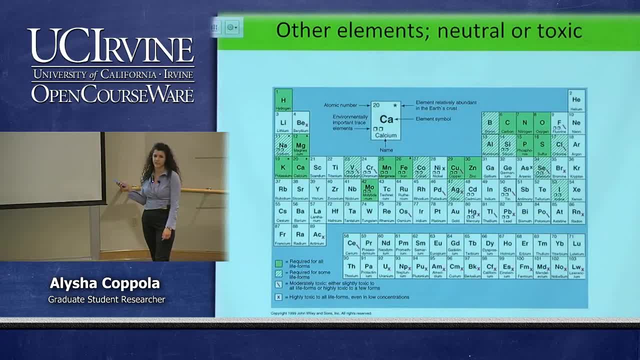 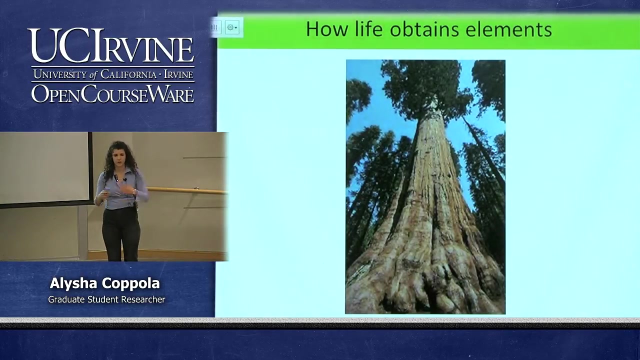 elements which are seen in their shaded white on the periodic table. those are carbon neutral. our may be needed in very small concentrations for some, but not all, or the can even be toxic and detrimental to the, to the organism. so for life to grow and to have energy. 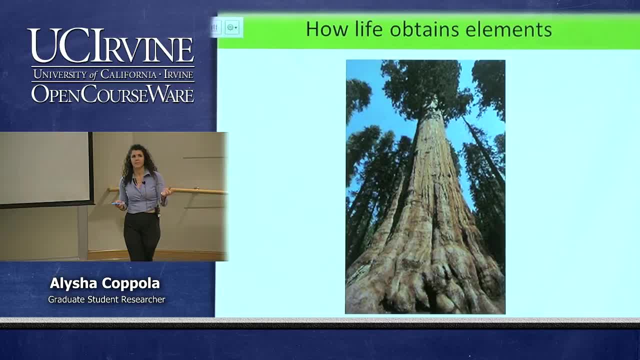 it needs the right amount of micron attraction, the right amount of macronutrients, supplied at the right time and in the right relative concentration of macronutrients 인 the right relative to each other. So has anyone seen one of these trees, or do they know what they're called? 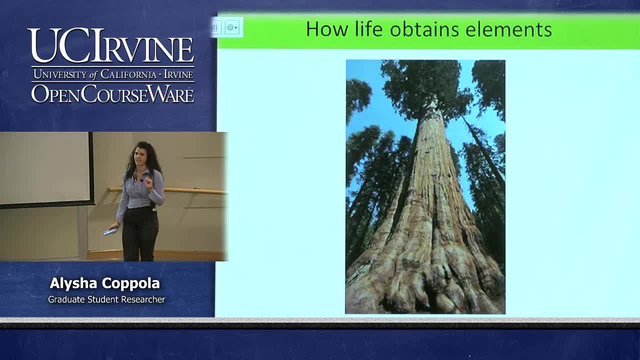 Sequoia. yeah, So they're huge and they're enormous and they go to like 300 feet tall and they have diameters of 50 feet, and the question is, how do they get all these nutrients from the atmosphere, biosphere and geosphere to create this huge, enormous structure? So I have an 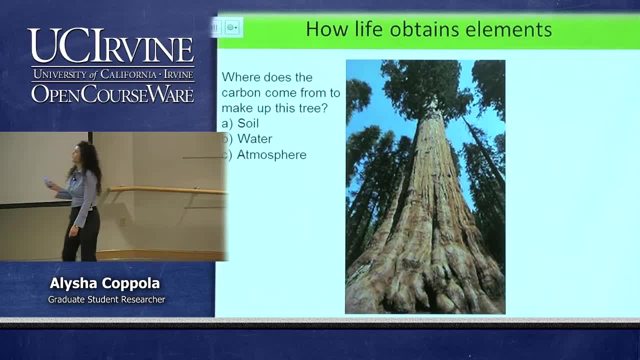 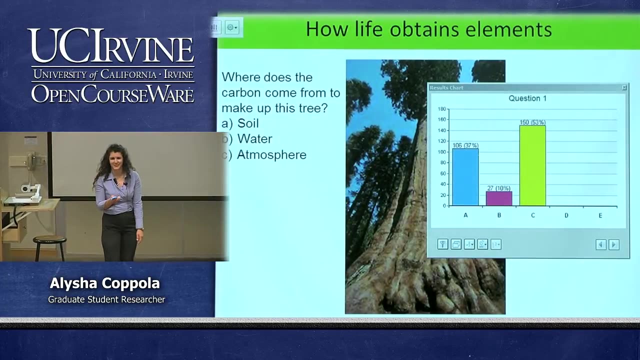 iClicker question for you guys. So where does carbon come from to make up this tree? So, does the carbon come from the soil, Does it come from the water, Or does the carbon come from the atmosphere? Okay, Okay, good, Everybody's doing a great job. So, yeah, the carbon comes. 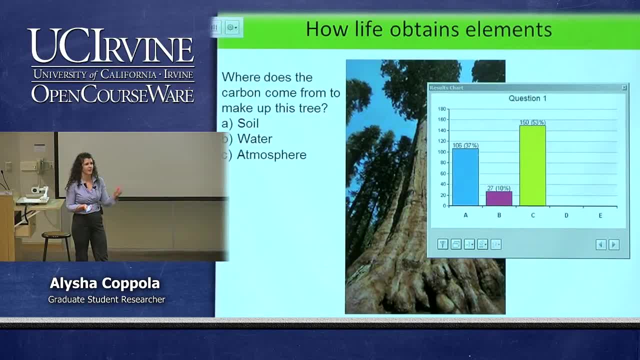 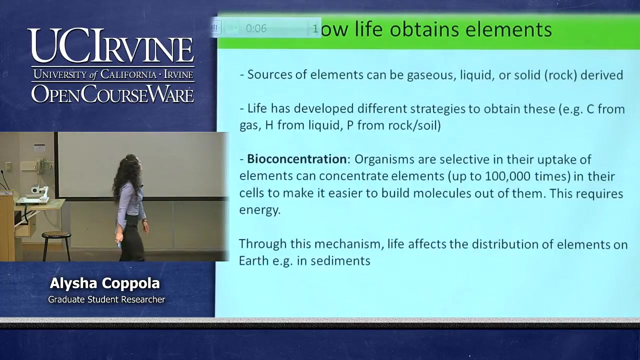 from the atmosphere, as you've through discussion, you see that carbon's incorporated through photosynthesis from the atmosphere and it's incredible that, given the atmosphere, it obtains enough carbon to build this enormous tree. so we're going to talk about how that – oops, Okay, we're going to talk about how that actually occurs. Oops, stop falling. 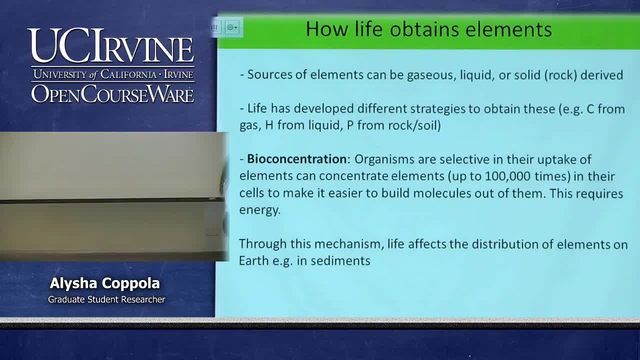 Okay, So we're going to talk about how that occurs, So the way that organisms actually, and life forms, vegetation and microbes are able to maintain photosynthesis and carbon sculpture. they're the first thing that happens. they're the first And for a謠. 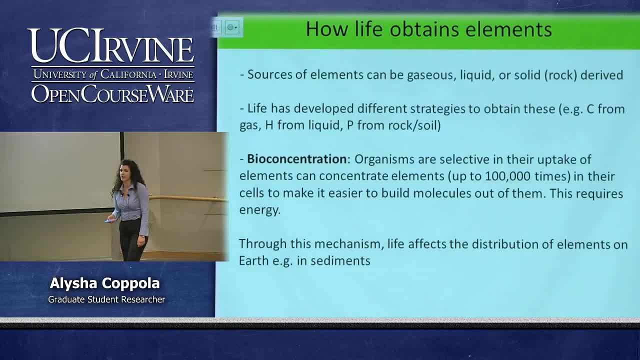 to get enough nutrients from their environment is to concentrate it. so that process is called bioconcentration and that's where organisms, selectively, are uptaking these macronutrients and micronutrients from their environment in higher concentrations to be able to grow, and sometimes this happens 100,000 times compared to its natural environment. so if you think, 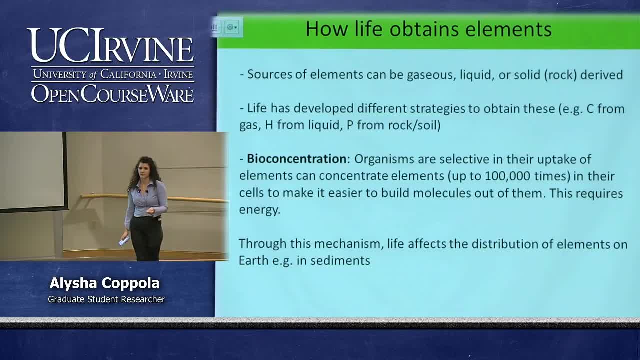 of algae, it can concentrate iron in concentrations 100,000 times than the sea water surrounds it, and this is where it's able to accumulate enough in order to grow, and so yeah, and then, through this mechanism, it ends up life, ends up impacting the environment and actually, 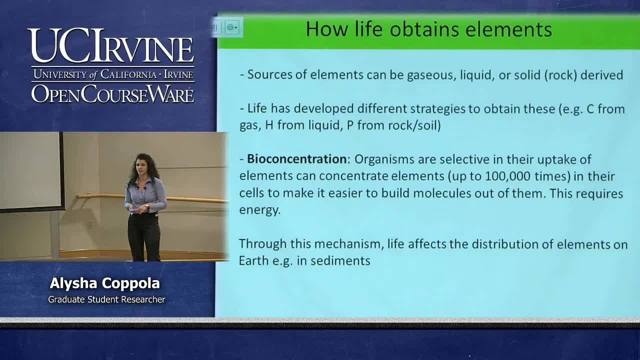 where the distribution of these elements are located. So, for instance, if you think of sea shells, so sea shells are grown in upwelling like skeletal remains. if you guys remember from the exam, there'll be a lot of skeletal remains falling down from the ocean because there's upwelling and a lot of calcium is incorporated into those. 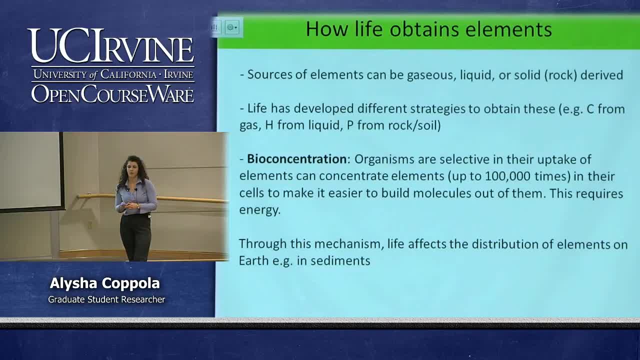 shells, so like coccolithophores or other organisms, can grow, and that will in turn affect the sedimentation and where calcium is formed or where it's formed, Okay. Okay, So if you think of phosphorus, it's present in organic matter and where those certain 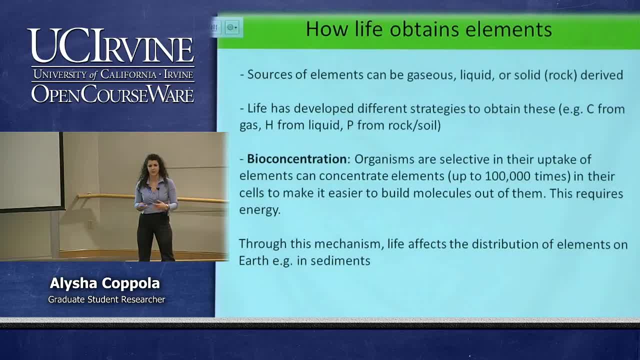 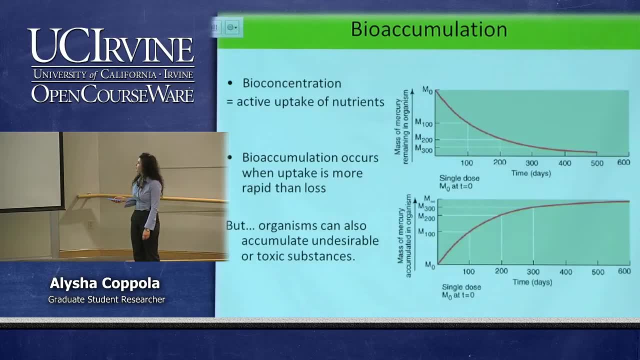 organisms are will ultimately influence where you find phosphorus and where it's deposited into the world's sediments. Okay, So, as we said before, bioconcentration is the active uptake of elements and nutrients, but accumulation occurs when you're adding nutrients more than you're being able to lose them. 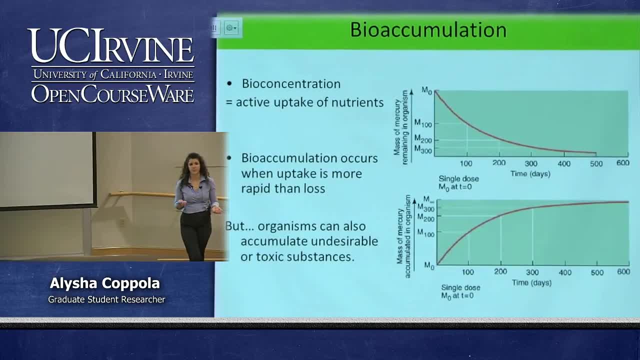 So, for instance, in the case of mercury, this is important because you're actually accumulating more and uptaking more than you're able to remove it from your body, for instance. So if you look at this first graph here, this shows on the y-axis the mass of mercury remaining in an organism, and if you give this organism one pulse of, 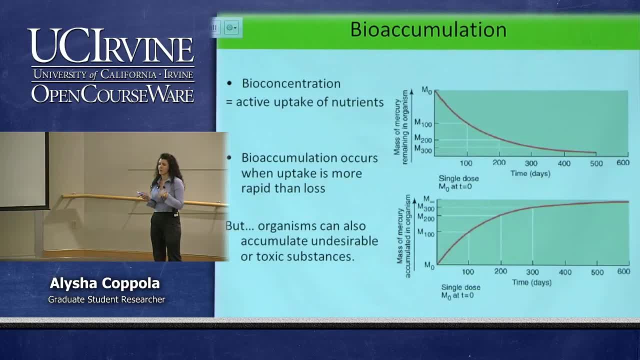 mercury, then it will start to decay so the body can remove it. so you only have one dose and you're not accumulating anything because your body is able to remove it. but if you're giving multiple doses and if you're, you know, for instance, eating small amounts of fish, 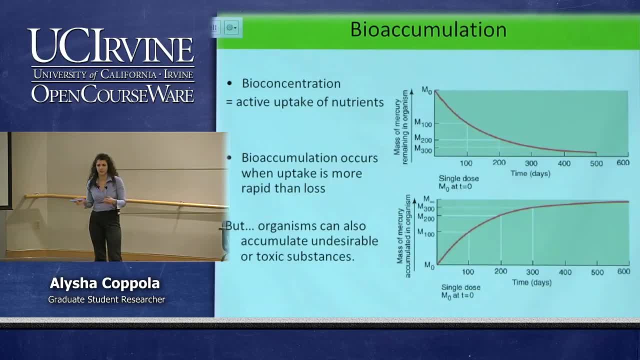 every day that have mercury in it. you're accumulating that mercury so you're not able to get rid of it. so that's why it ends up that you're accumulating this mercury in the organism. so this is important in instances with fish and also in the rest of the biosphere, where 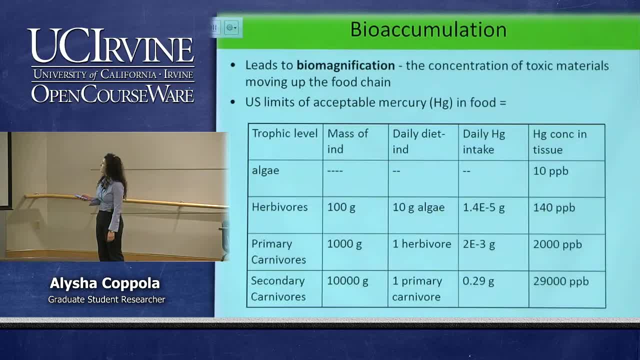 you can accumulate these elements in your body. so this bioaccumulation leads to biomagnification, and that's where you a lower trophic level- for instance, algae is accumulating mercury of 10 parts per billion- and then higher trophic levels- herbivores. 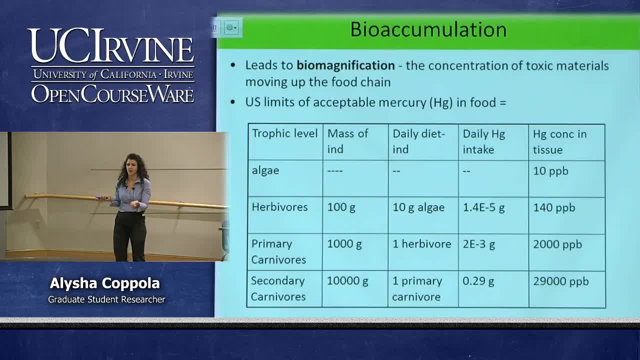 will eat the algae and accumulate an even greater amount of mercury in it, and then the concentration increases more and more as you move higher up the trophic level. so then, in a secondary carnivore- if it, you know, survives that long with all that mercury in it can get, can contain concentrations. 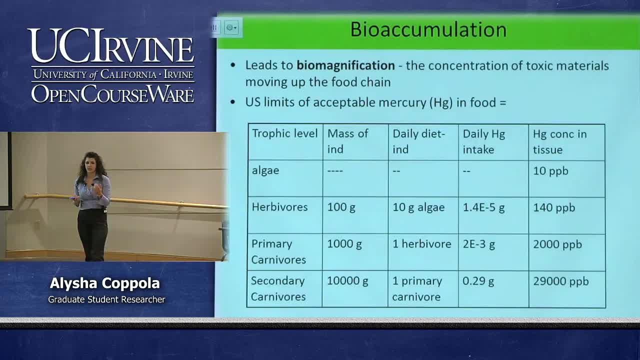 of 29,000 parts per billion in it, and that's where you can actually accumulate and magnify the amount of mercury that's present in the ocean water into these organisms. so does anyone know what the US limits of mercury in food is? can you just throw out a guess? 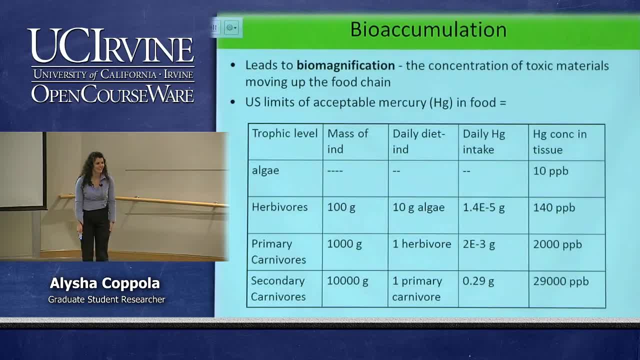 yeah, I have a feeling you have an answer. yeah, so it's close, it's 50, so so that's pretty, that's pretty, that's pretty surprising. so that's why it's important to actually eat fish, not very often, and they sometimes say pregnant women shouldn't have fish. and if 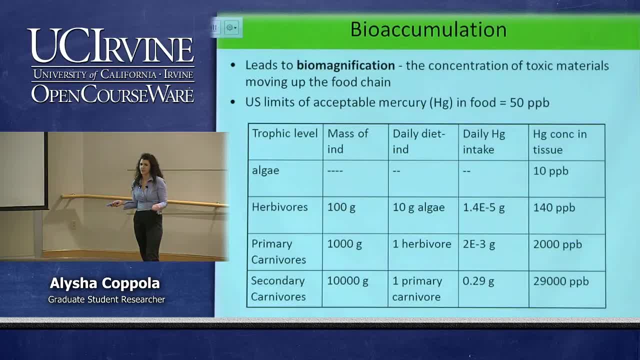 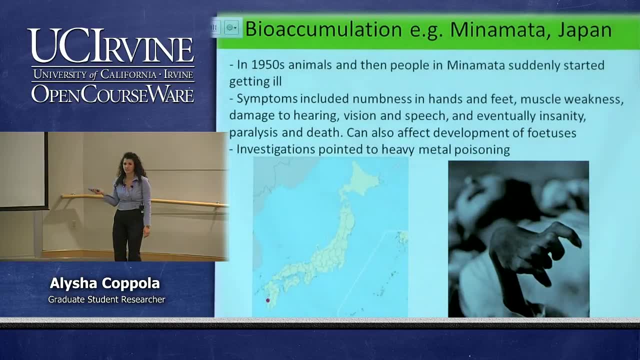 because you don't want this accumulation of mercury as you move higher up in trophic levels. So this was important in Minamata, Japan in the 1950s, where they found a lot of toxicity among the central nervous system of these habitants of Minamata Japan. 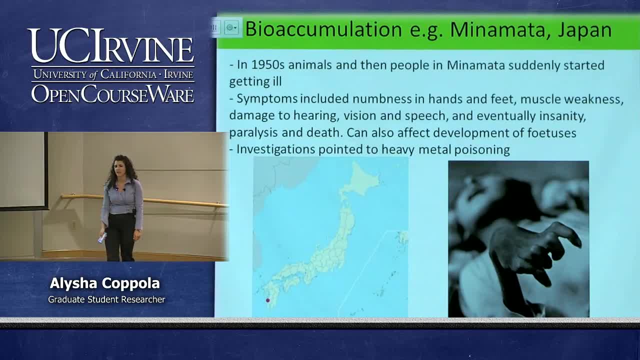 And this was mostly fishermen and their families were getting severely ill and they had numbness in their hands and feet. They were losing their hearing, their vision and speech, and it ultimately led to death. So investigations thought this was heavy metal poisoning and what they found is actually there was a power plant. 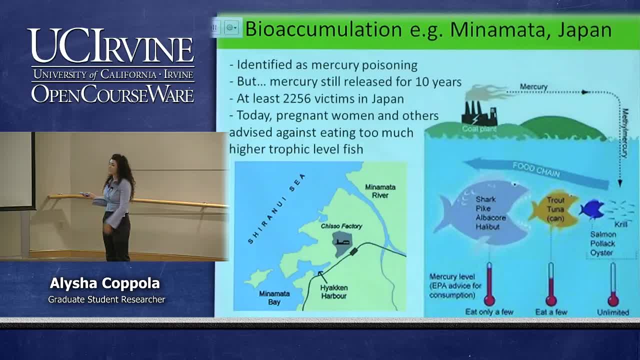 producing plastics that were releasing mercury salts, that were producing mercury salts, that were producing mercury salts. They were using it in the chemical processing of these plastics and they were getting washed out and depositing into the ocean And then into the ocean, even though they were lower concentrations. 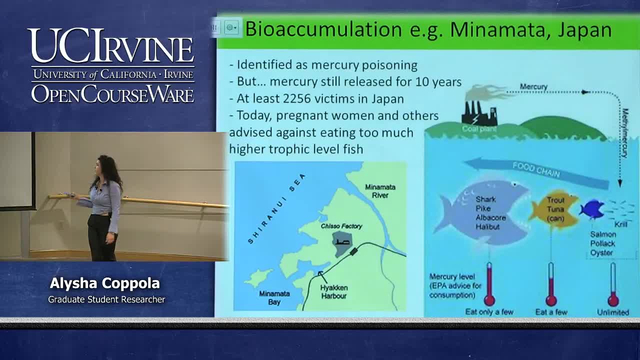 they were accumulating in each level, each trophic level. So the krill would have levels of mercury, but then, as each trophic level would eat the krill, it would be more and more concentrated until, ultimately, the fishermen and their families were eating this. 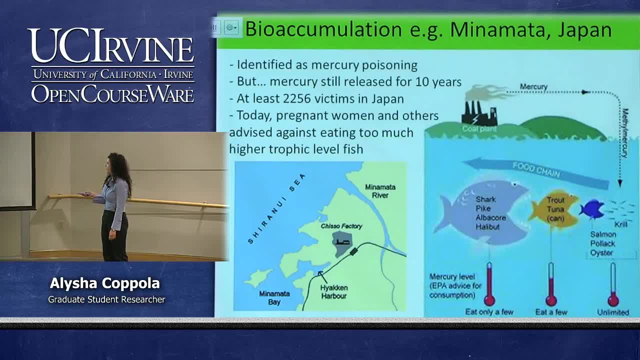 And so they were able to eat this fish that was highly toxic, So that's why I put this link for the Monterey Bay Aquarium. They have a seafood watch, and that's why it's important to check which seafood you're eating and if it's sustainable. 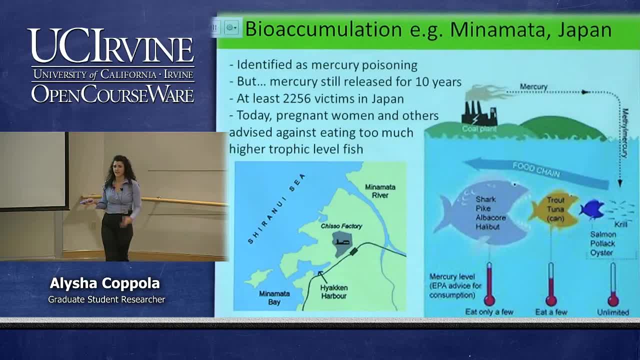 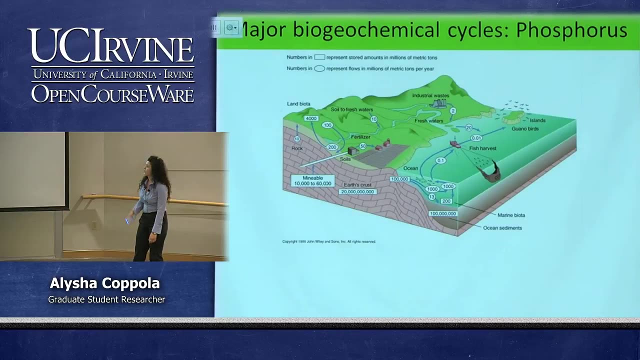 and also the EPA also advises how much of certain fish to eat. So that's why you want to eat lower in the trophic level. Does anyone have any questions? Okay, So now we're going to talk about one of the major biogeochemical cycles, and that's phosphorus. 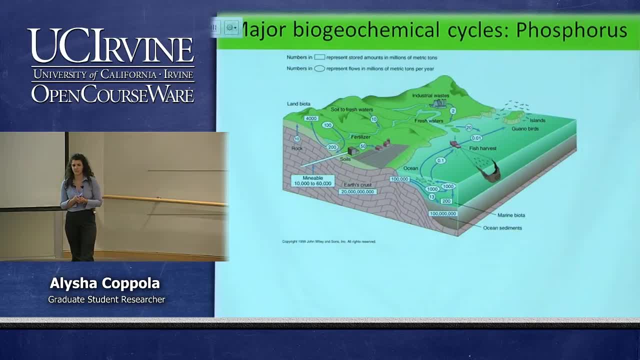 This is required for life and it's one of the main limiting reagents for vegetation. So most so in the boxes. it shows the stored amounts in millions of metric tons. So In the soils, in the earth's crust, that's where you have most. 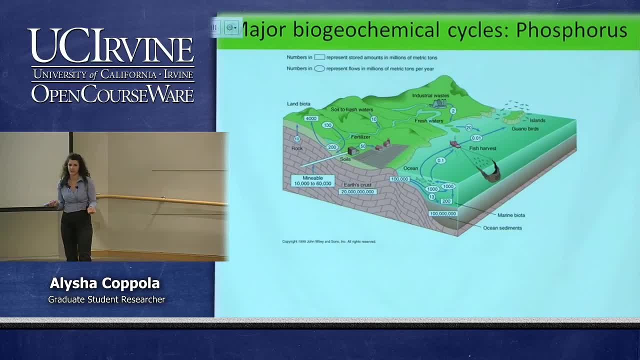 of your phosphorus, and the phosphorus isn't usable to the rest of the biosphere unless it's in the form of phosphate for it, so it can be usable for these organisms to incorporate into their bodies. And the way you get phosphate out of phosphorus is: 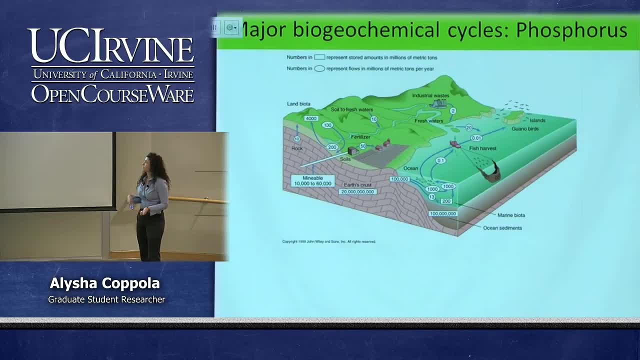 by chemical weathering of these rocks. So then that will be, the phosphate will be used on land and vegetation and then also it will run off into the ocean and increase productivity in the marine life. So you'll have it will impact the ocean biota. 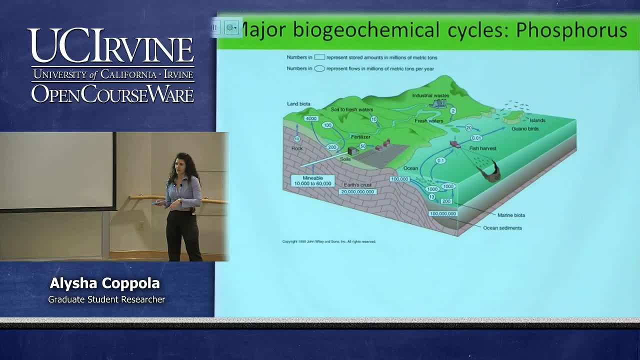 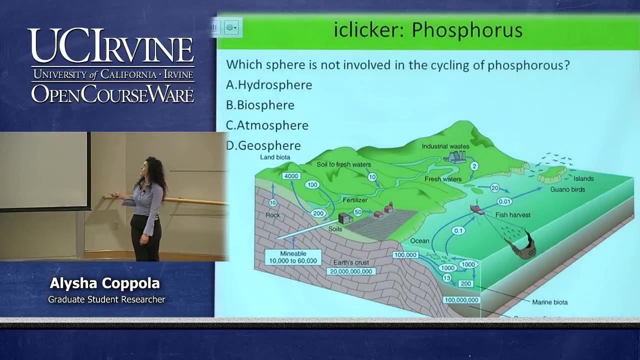 and then it will, eventually these organisms will die and it will eventually go into the ocean sediments and then again these ocean sediments, under pressure, will form more of earth's crust. So my question for you today is which of the sphere involves is not involved? 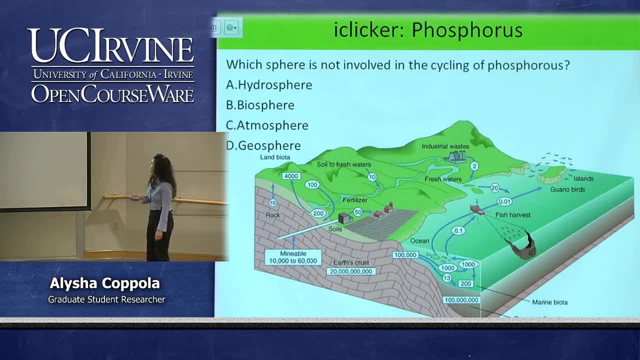 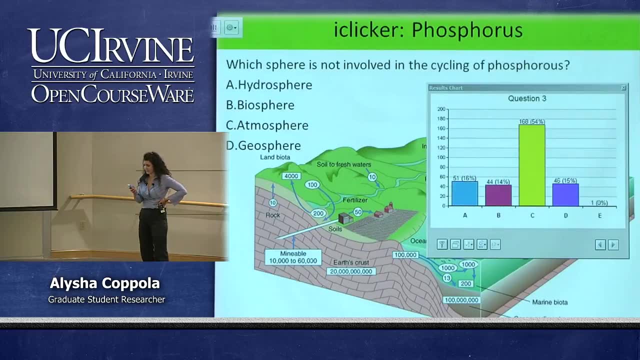 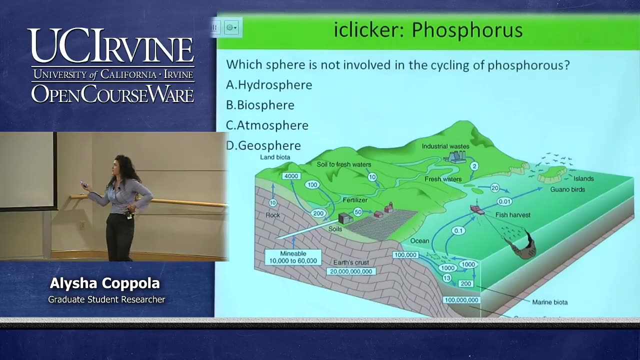 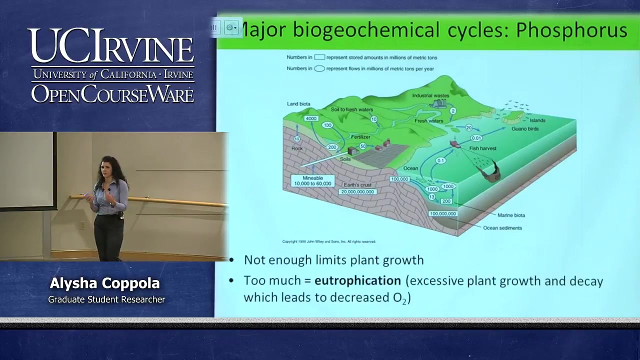 in the cycling of phosphorus, Okay, good. Yeah, the atmosphere is not involved in this cycle, So phosphate is washed out into the ocean and then deposited into the sediments, and it doesn't involve transport by wind into the atmosphere, And so, like I said before, it's very important for plant growth. 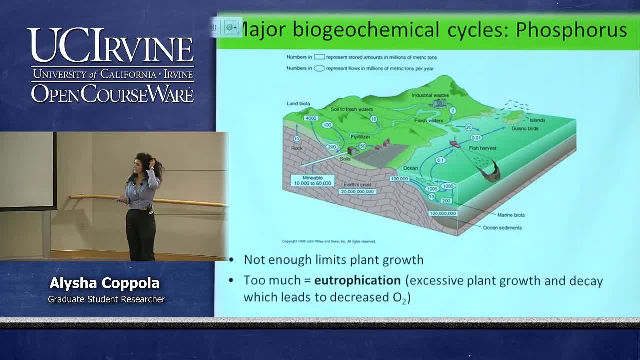 to have a lot of phosphate so it can grow, And if you don't have enough, this will often be the limiting nutrient for growth. However, if you have too much, it can lead to eutrophication, where you actually end up having excessive plant growth. 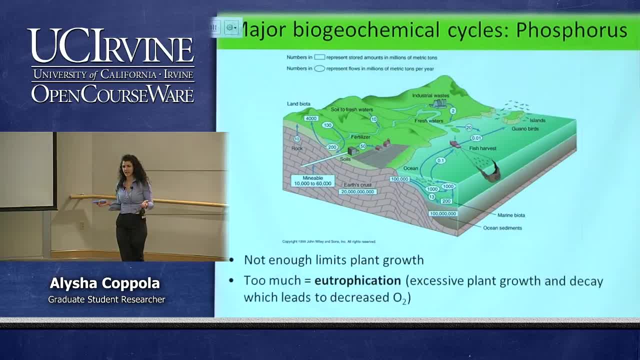 so you'll have blooms, like in the ocean of all this marine life, and because of these blooms they'll be using a lot of oxygen and creating these oxygen dead zones. So it will be hard for fish to live, and that's when you get a lot of fish kills. 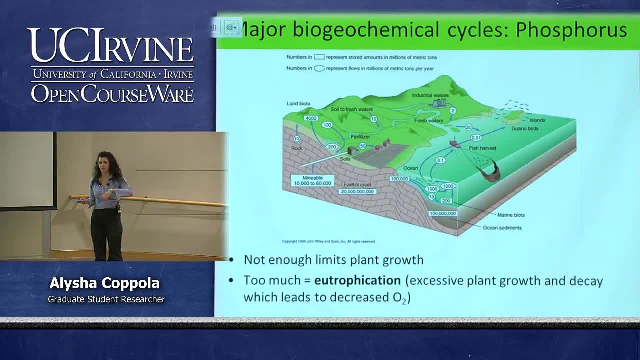 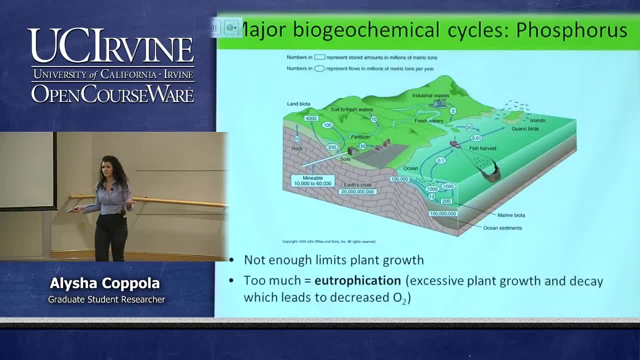 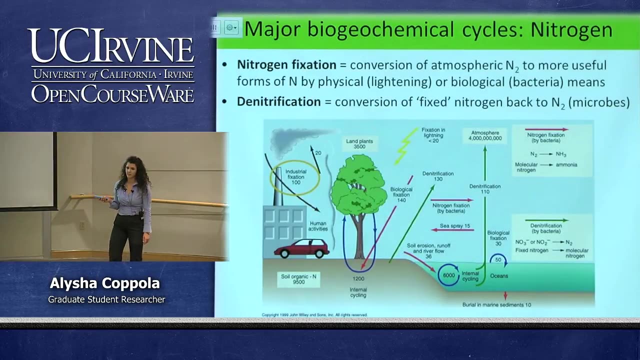 Yeah, Yeah, Yeah Yeah, Fertilizer, exactly. So we want things to grow to support our community and our population, so we add excessive fertilizer to our lands that end up running off into the ocean. So yeah, So one of the other biogeochemical cycles? we'll look. 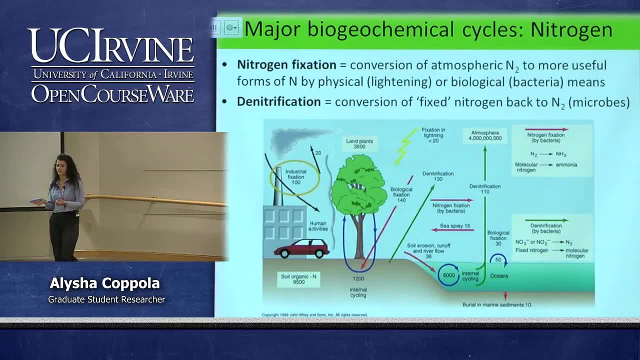 at is the nitrogen cycle, and this also, like phosphorous phosphate, is very important for growth and is often a limiting nutrient factor in plant growth. So does anyone remember from studying for midterms and exams the percent composition of nitrogen in the atmosphere? Yeah, so 78%. so even though nitrogen is present in 78% in the atmosphere, it's often limiting. 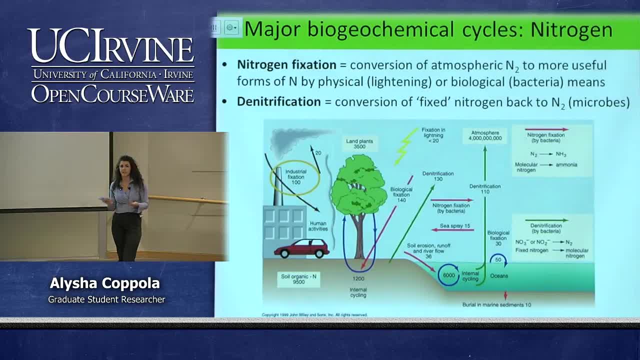 for plant growth, and the reason that is is because N2 in the atmosphere is not very usable by marine life, so it's relatively inert, the nitrogen in the atmosphere. So the way that this N2 from the atmosphere becomes usable to life in organisms is from. 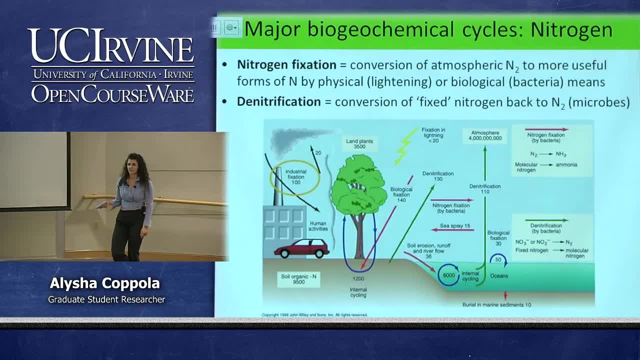 the conversion of N2 to nitrate or other forms of nitrogen. We call it fixed nitrogen that organisms in life can take up. So one way that occurs this process of nitrogen fixation is through lightning. So lightning Lightning accounts for about 10% of all the fixed nitrogen on earth and the other 90% 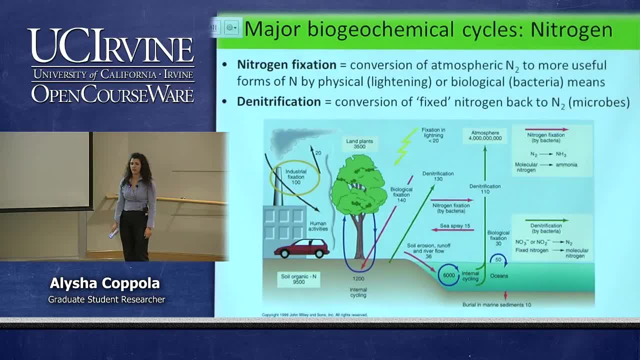 is from microbes, So microbes in the soil, converting this N2 into this usable form of nitrate. So that's what you see here in this red arrow: from the atmosphere into the soils. So that's where you get that usable nitrogen And that's used in formation of land. 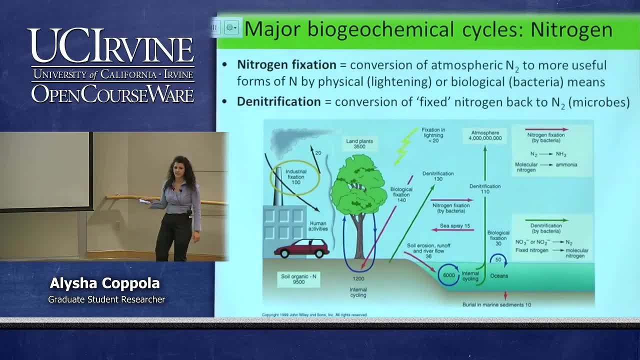 Formation of land plants. It's also that fixed nitrogen washes out to the ocean and is used in the marine ecosystems and helps the marine organisms grow and the phytoplankton and plants in the ocean, And then is deposited into sediments and recycled. 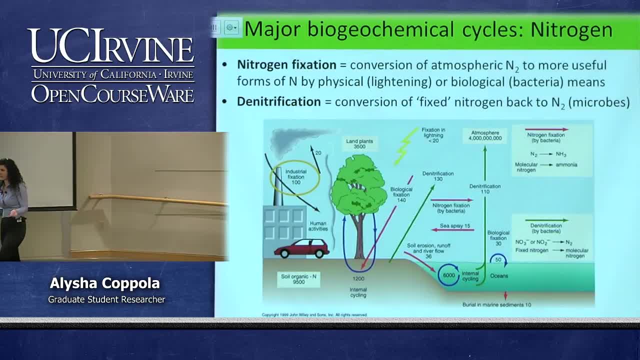 Denitrification is the process where that nitrate is converted back to N2 and released back into the atmosphere. So, as you can see here, this is a, if you wait for lightning and microbes to occur, this is a really slow process and that's why the natural cycle would be is limited by 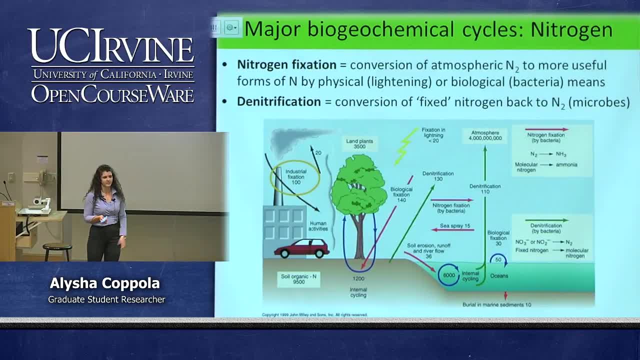 microbes and this, these N fix, these nitrogen fixation processes. but we came up with this chemical reaction, the Haber process, that's able to use nitrogen from the atmosphere to create nitrate, And this is important for fertilizer and growing our crops. 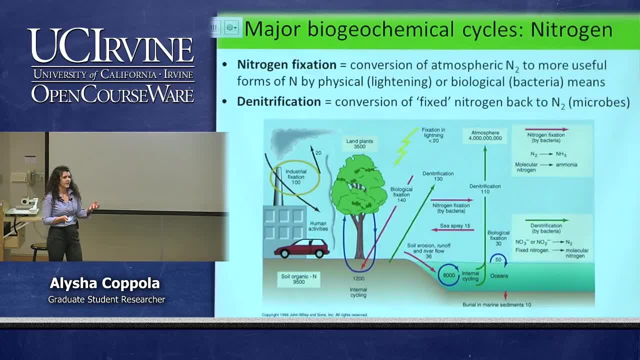 So in this way we've altered the cycle because, like phosphate, where you're limited by the erosion of phosphorus in the rocks, you're limited by these microbes. but we've altered that cycle by providing excessive amounts of nitrate to the ecosystem. 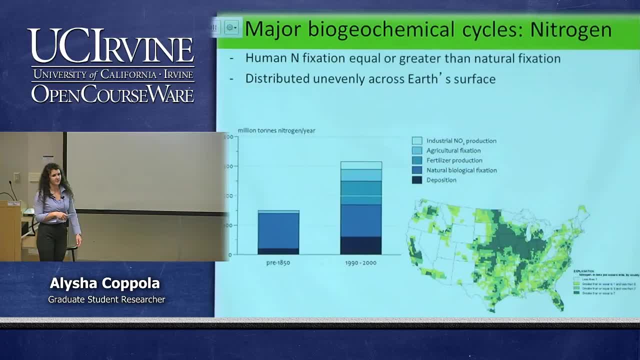 So this figure shows in the pre-1850s- Okay, In the late 1850s- how much nitrogen was available, and most of it was through natural biological fixation. and we've since doubled that since the 1900s, by actually producing nitrate. 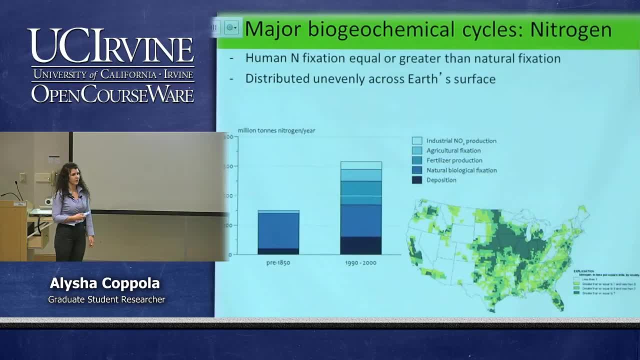 And most of this nitrate ends up in areas where we grow. So in the central of the US, where we have a lot of crops, we'll apply this fertilizer so we can grow enough and there won't be any limitations on growth. and quite often too much is applied and it will run off and be. 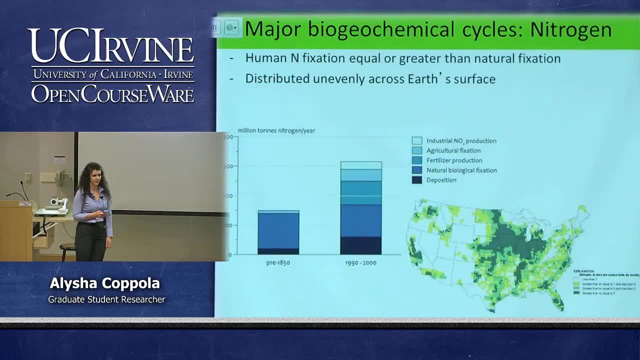 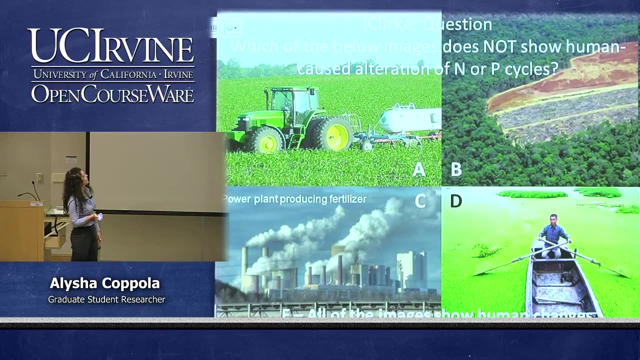 distributed, but most of it is concentrated where we have a lot of growing. Does anyone have any questions? Okay, So which of the below images does not show human-caused alteration of the nitrogen or phosphorus cycles? Okay, So let's look at this. 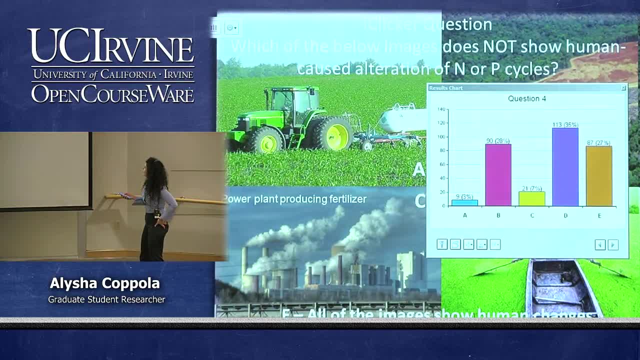 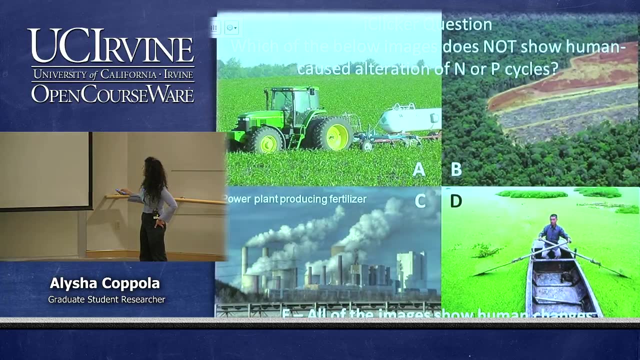 Okay, Let's look at the results. Okay, So, yes, So, actually, so, E is the correct answer. All of them show human influences Head graph. So actually, D is an example of eutrophication, So that's where you have a lot of phosphate into the ocean and or into streams and lakes. 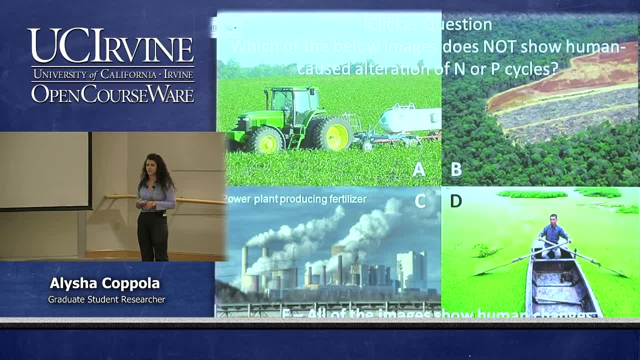 and what you have is excessive nitrate And so the eutrophication. you know you have biologic nitrogen as a form of nitrogen, and so this is an example of the natural cycle where you have a lot of nitrate. You almost don't have it on the surface, it's just a little bit of a liked material. 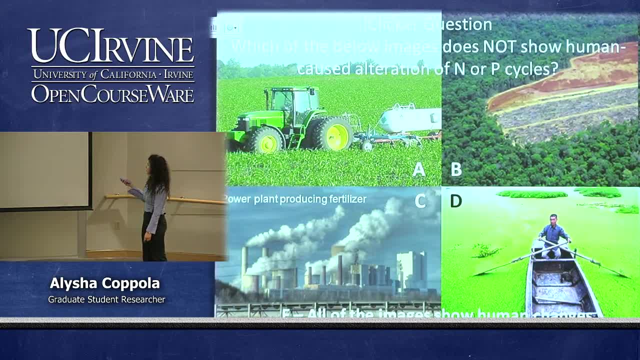 D is a little bit of a liquid. So what we can see here is that, if you see, if you see this out, Okay, Here's your nitrogen And that's what you have- a lot of nitrogen, Okay. So if you look here, you can see if you're looking at this image, that's you know. 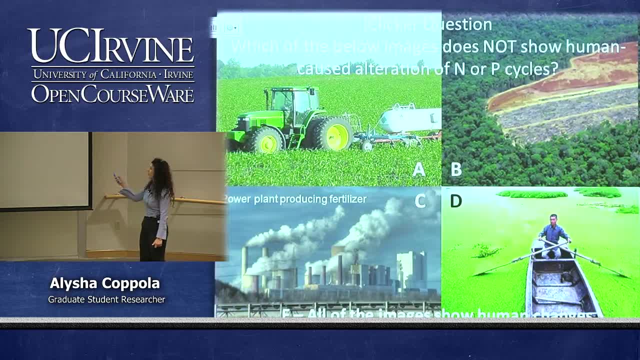 something that we call a carbon per year satisfy. Okay. Now if you see, if you do the scientific and you see that it has a carbon per year, and you have a carbon per year and you've got a carbon per year, but it's a carbon per year. 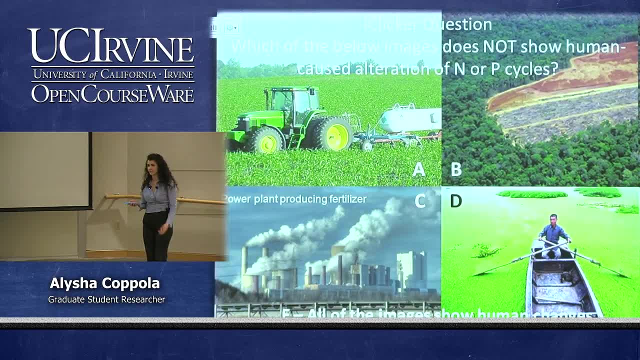 of them have actually altered the natural cycles And if you look at anything, the human fingerprints on all of these biogeochemical cycles have been altered from the industrial revolution and putting CO2 into the atmosphere and, you know, creating these usable forms. 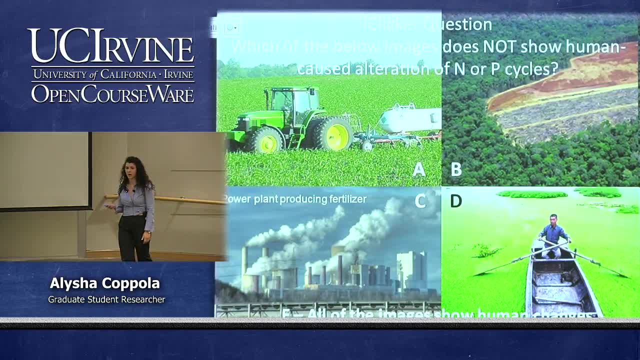 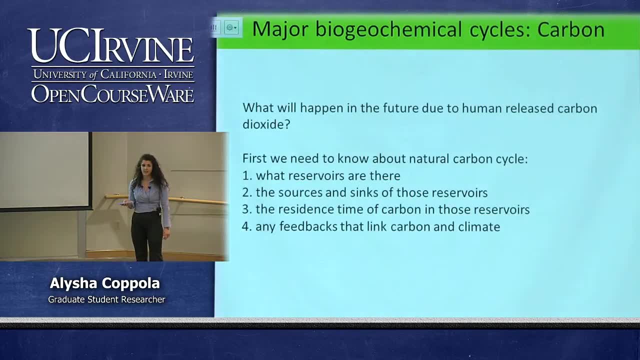 of nitrogen and phosphate that we're often limiting in other areas. Okay, So one of the major things that we're interested in is understanding what will happen in the future due to these human influences that we've definitely altered. So first we need to understand the natural carbon cycle. 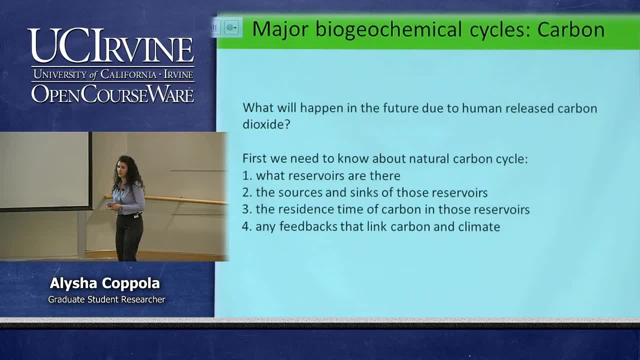 So we need to know what the reservoirs are. So where is the carbon stored, What the soil is, What the sources and sinks are in those reservoirs. So how is carbon added to those reservoirs and how is it taken away? 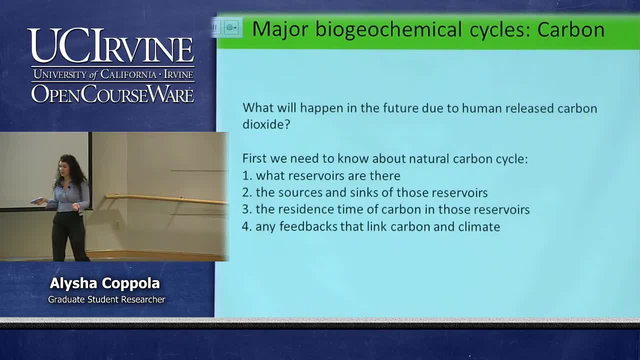 What the residence time of carbon in those reservoirs are. So how long has the carbon been there? And then also any feedbacks that link carbon to climate. So, like we've talked before about how you can have a positive or negative of feedback and how 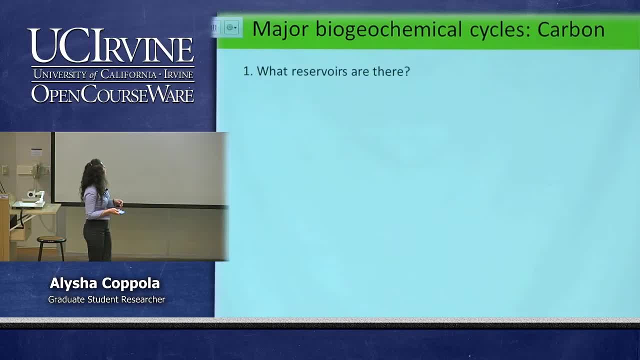 that will influence these reservoirs. So can anyone come up with? just name a couple of carbon reservoirs, or one is fine. So what is a container of carbon? What was that? Yeah, the ocean. The ocean is a carbon reservoir. 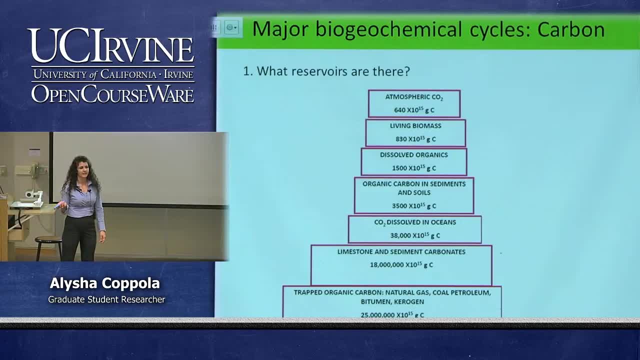 And actually the ocean has as much carbon as the atmosphere, which is very interesting, And organic carbon, So the atmosphere contains a lot of carbon. About 45% of carbon is in the atmosphere. About 25% is absorbed into the oceans. 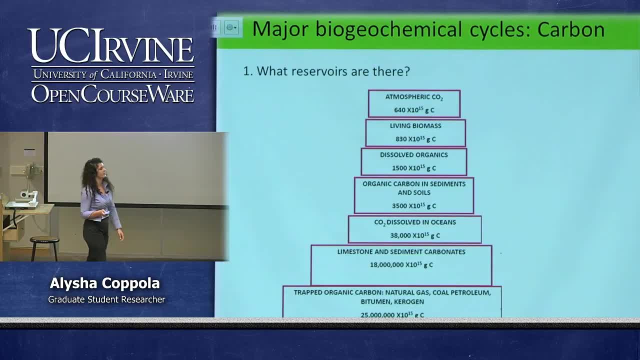 And about 30% is into the terrestrial biosphere And atmospheric CO2 and the terrestrial biosphere and dissolved organics- that's dissolved organic matter from things decaying- are some of the shorter reservoirs. We also have organic carbon in soil and sediments. 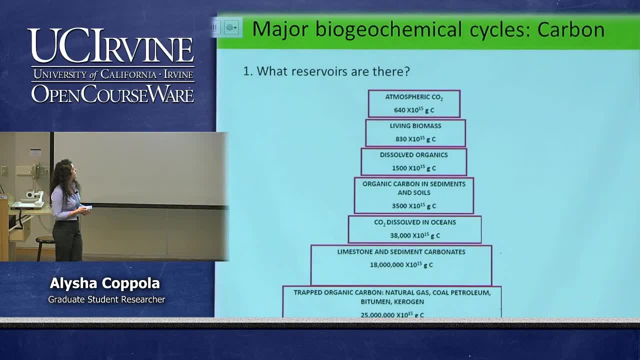 And that includes things, yeah, like permafrost, that are frozen solid earth. We also have CO2 dissolved in the ocean, So that's CO2 in the atmosphere interacting with the ocean and dissolving within, So that's called inorganic carbon. 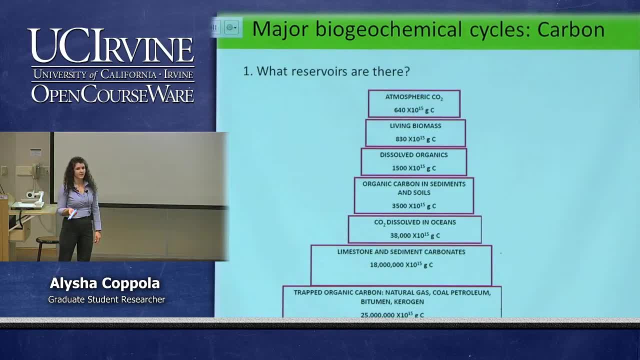 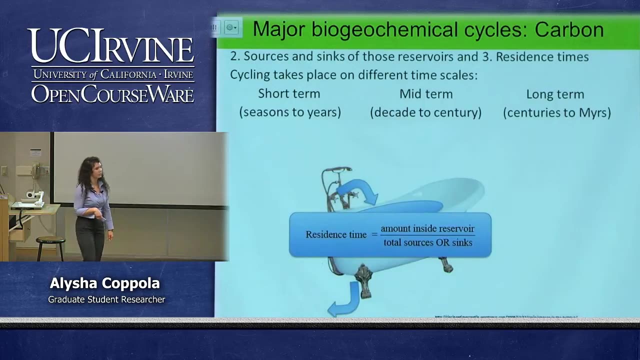 We have carbon that's present in limestone and sediment carbonates, And then we also have trapped organic carbon, which is where we get our fossil fuels from petroleum kerogen. And when we want to know these residence times of these certain reservoirs or how they respond? 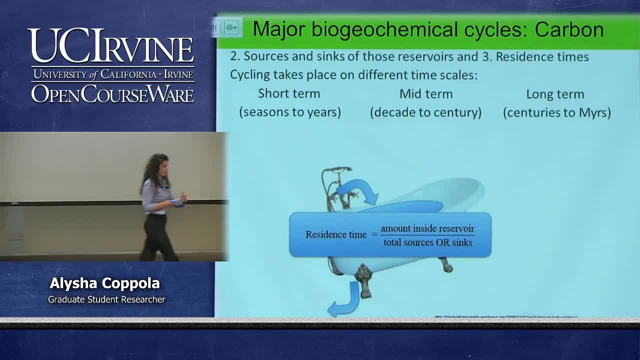 and how quickly the carbon is contained in those reservoirs or how long they've stayed there. we look at residence time, which is the amount inside the reservoir over the total sources or sinks. So, like we've talked about before, with this tub 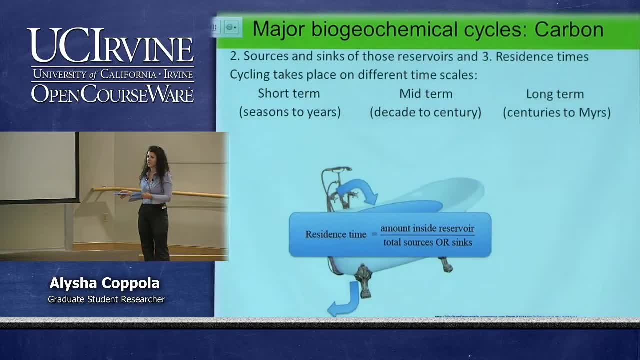 how much water is in the reservoir and how much is removed by. you know either a leak or is being added. So that's how we can determine the residence time of these large reservoirs and how they may respond. So they cycle the carbon in these reservoirs. 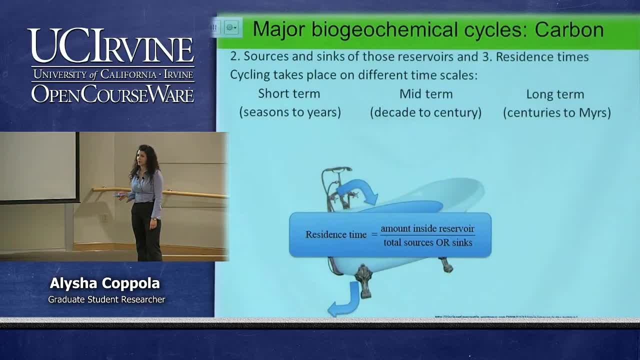 that I just showed you Cycle on different timescales, So the carbon in the atmosphere will respond differently and cycle on a different timescale than the carbon in that is contained in sediments, for instance, So they can be short-term, from seasons to years. 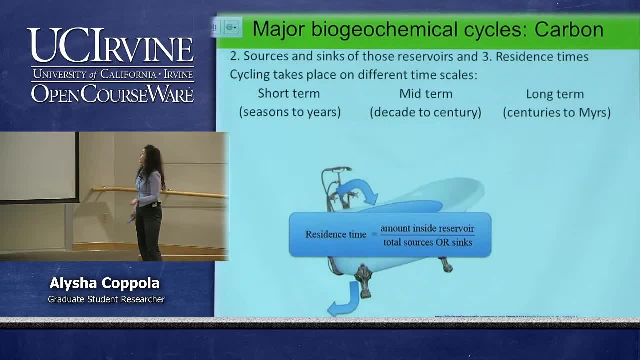 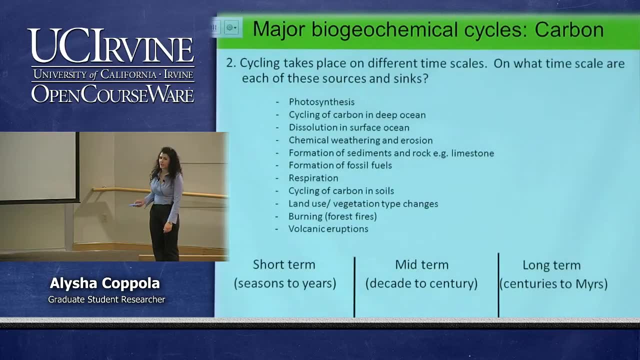 They can be mid-term, from decades to centuries, or they can be long-term, from centuries to millions of years. So you guys can talk about this. I'm going to give you a little bit of time, Talk amongst yourselves, and what I've done here is put. 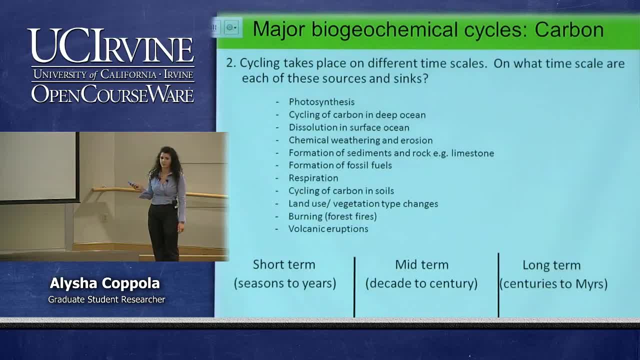 up a list of each of these carbon sources and sinks and that occur on Earth and you guys can break up into groups or talk amongst yourselves and put these different sources and sinks and organize them between short-term, mid-term and long-term timescales of cycling. 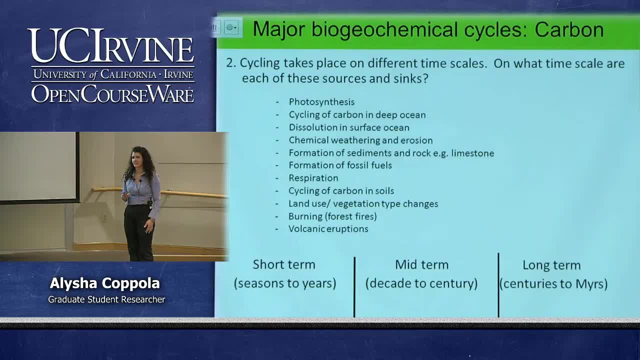 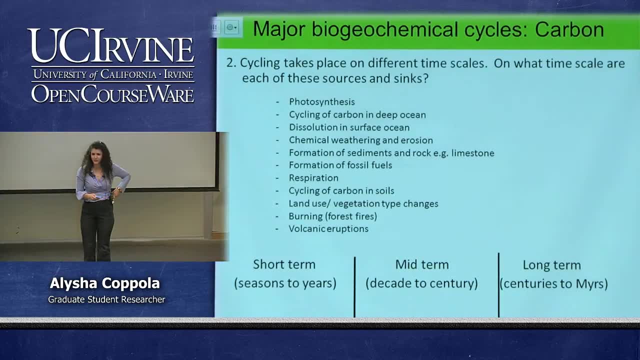 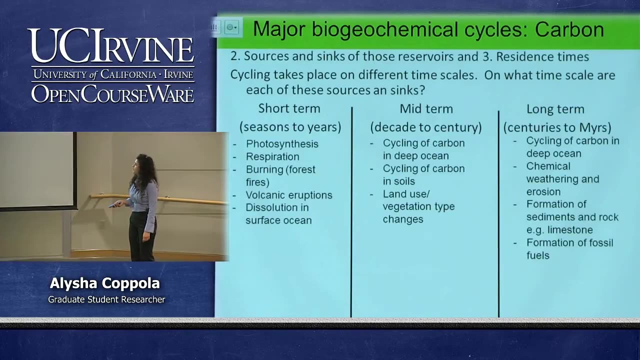 So, and I guess we'll walk around and help you guys with any questions. So it seems like everyone is it on, So it seems like everyone had some really good discussions and conversations about this. So when we're talking short-term of seasons to years- 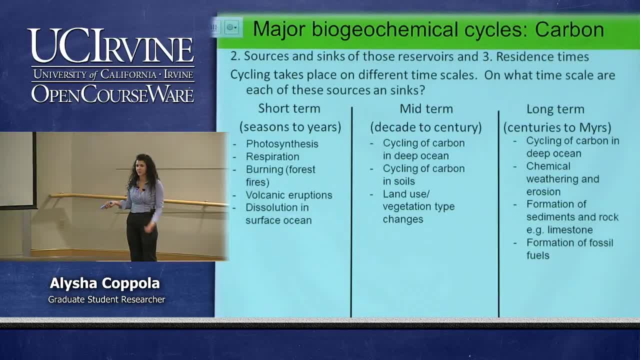 that would be something like photosynthesis and respiration, where it's up-taking CO2 and it's on much shorter timescales than something, for instance, like cycling of carbon in the deep. So, if you remember, back to the deep ocean circulation. 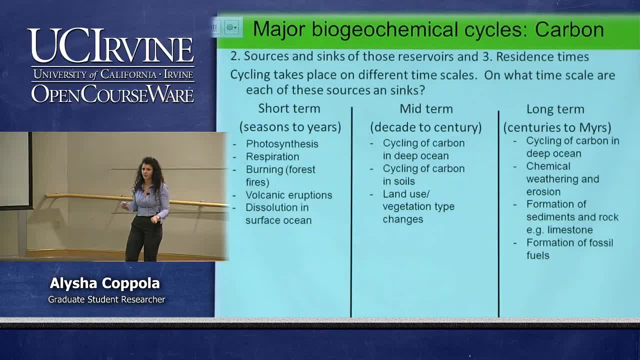 you have water sinking through the formation of this North Atlantic deep water, because it's getting cold and salty and it's sinking and it's traversing around the entire globe and then resurfacing in the North Central Pacific, not Central the North Pacific, and that's a much longer timescale. 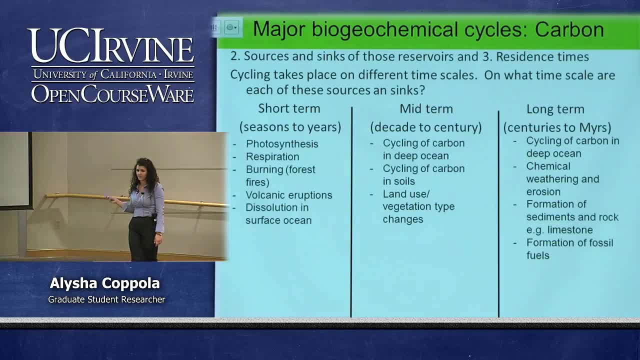 That's 1,000 years. so that's that carbon is going to be tied away for 1,000 years, opposed to to carbon that's in trees- much shorter timescales. you know when you have a forest fire or the tree dies and is decomposed. 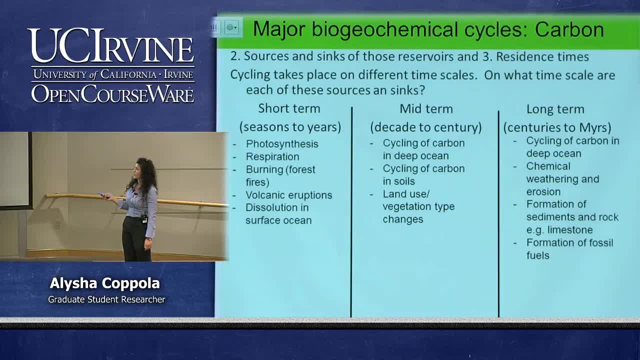 So. so other short timescales is burning of forest fires, volcanic eruptions, dissolution in the surface ocean. Mid-term timescales of carbon cycling: is this 1,000 years for cycling of carbon? Cycling of carbon in soils is also on intermediate timescales. 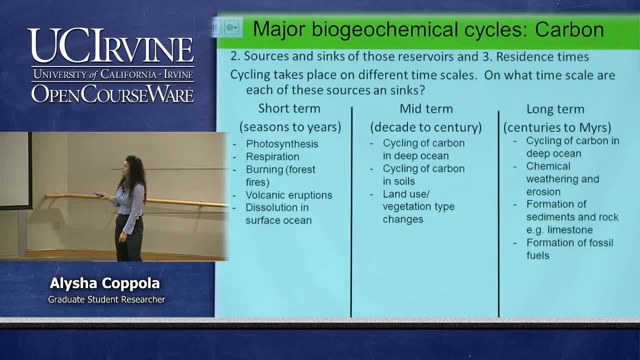 and land use and vegetation changes. Our longer timescale changes are cycling of carbon in the deep ocean, the chemical weathering and erosion of rocks, formation of sediments and rocks, and then formation of our fossil fuels, which take a long time. So the different sources and sinks of carbon are very important. 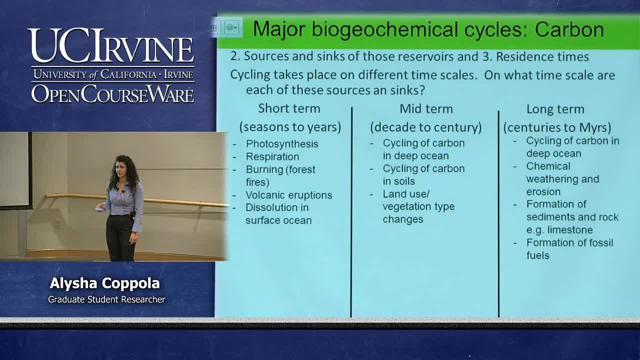 and also their residence time within these pools are important to understand the natural carbon system, so we can understand how things may change when we're adding more carbon to the system by burning this fossil fuel, And it's like we've talked before when we've talked. 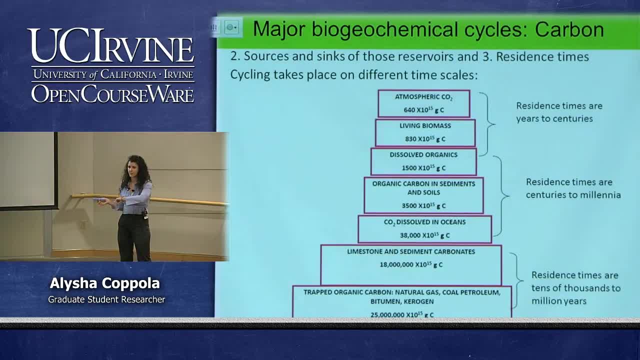 about earth being a closed system. you can't take carbon from fossil fuels. You can't burn fossil fuels and not have it show up someplace else. So when we're burning fossil fuels, it's showing up in the atmosphere and in one system all of them are affected. 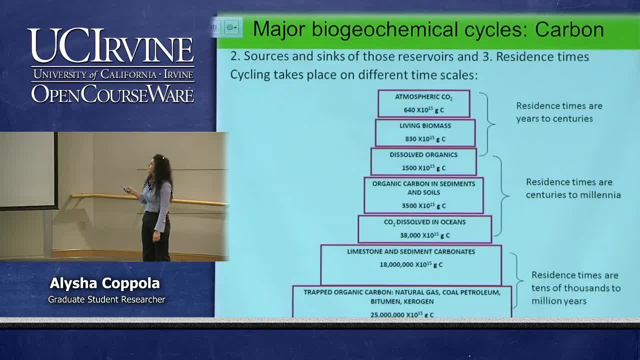 So do you see here, the smaller reservoirs have the shortest residence times, whereas the residence times are centuries to millennials for these intermediate carbon pools. and the larger the carbon pool, the slower residence time it has, so the slower it takes to change these pools. 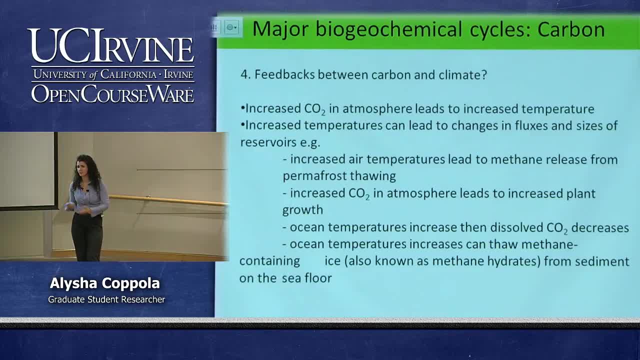 So now we're going to talk about feedbacks within these carbon pools and how those change climate, whether they're a positive or negative feedback. So we're increasing CO2 concentrations into the atmosphere and that's leading to increased temperatures because it's a greenhouse gas. 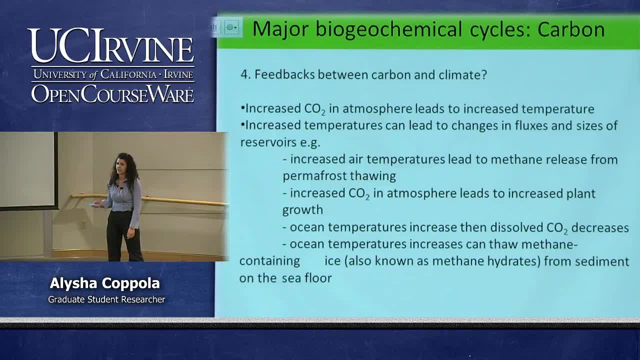 And these increased temperatures increase the fluxes and exchanges between those other reservoirs that I just showed on the previous slide. So some examples of this is: increased air temperatures lead to methane release from permafrost thawing, So permafrost is located up north, in the northern latitudes. 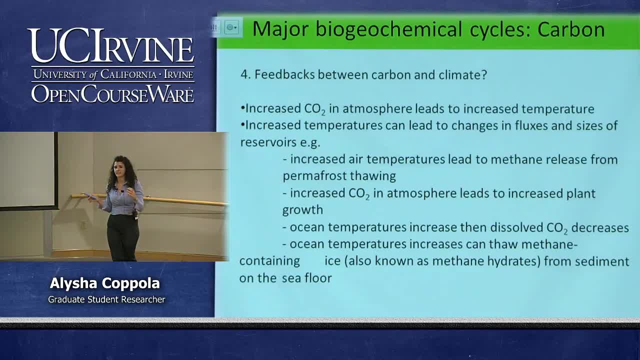 and it's this soil that's been frozen and it contains a lot of carbon and it's a large carbon pool. But as we're increasing temperatures, this permafrost is starting to thaw and microbes are getting involved in it and decomposing and you're releasing, making some. 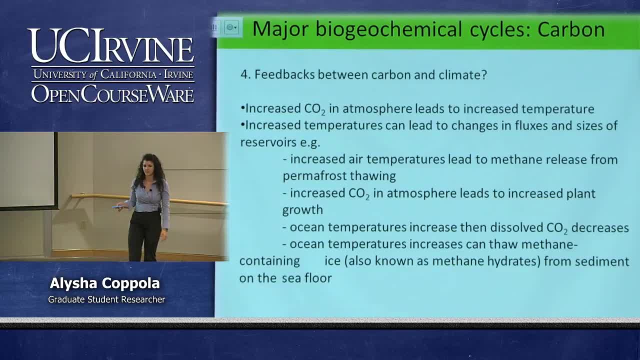 of that previously frozen carbon now available to the ecosystem. Another example is: increased CO2 in the atmosphere leads to increased plant growth through photosynthesis. So you have more CO2 in the atmosphere, so it's easier for plant stomatas to uptake this CO2. 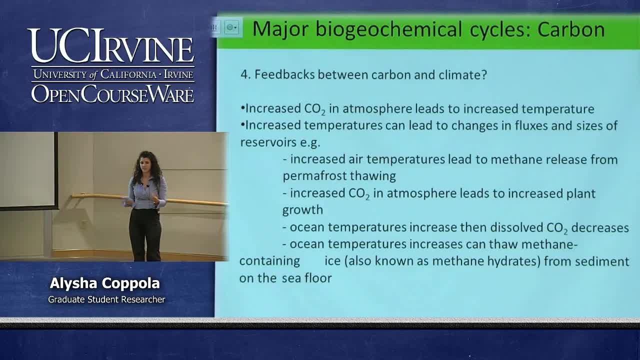 for photosynthesis, like we talked about in your discussion. So you're actually requiring CO2 for photosynthesis, and if there's more CO2, it's easier for plants to grow- And that's called CO2 fertilization- And ocean temperatures increase, so then the amount of CO2 dissolved. 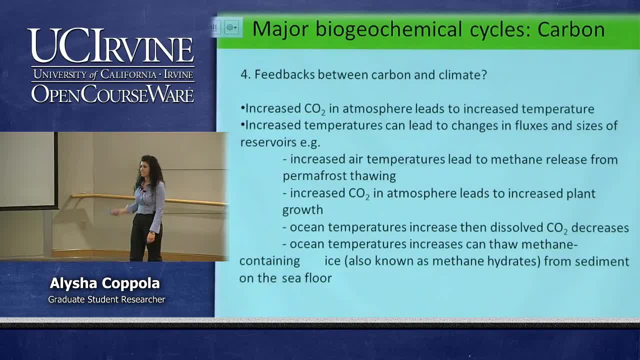 in oceans actually decrease. So if you think of a can of soda on a hot day, if you open the can of soda and let it sit out, what will happen to it? Will it be really tasty, you know, or you know? 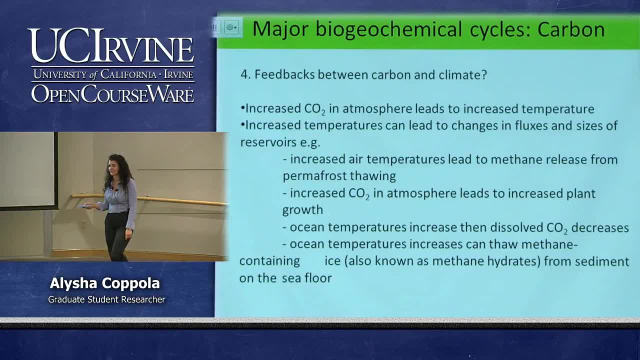 something not very good. Yeah, so it will be flat because the CO2, it's easier to dissolve CO2 into colder temperature liquids And then ocean temperatures, Temperatures increase and this can thaw methane-containing ice which is located in continental shelves. 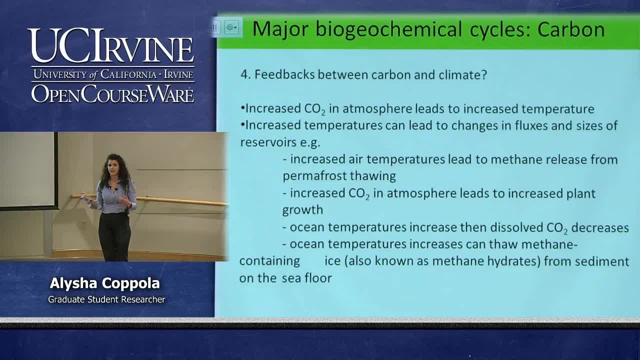 So the ocean temperature will be warmer and it will start to release the methane that's contained in these areas of ice under the ocean, And they're also known as methane hydrates. So let's talk a little bit in more detail about each. 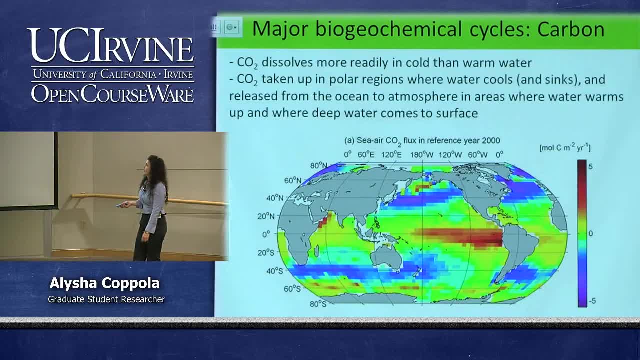 of these feedbacks in the carbon cycle that we're interested in. So CO2.. It dissolves more readily in colder waters, So as you can see here. so this is a figure of the amount of air-sea CO2 flux. 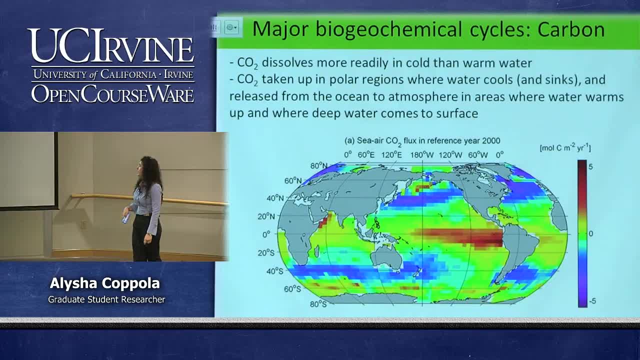 So that's the amount of CO2 that's being drawn into the ocean. So the purple-bluish colors represent where you're withdrawing or you're drawing in a lot of CO2 into the ocean, So you're taking a lot of CO2 from the atmosphere. 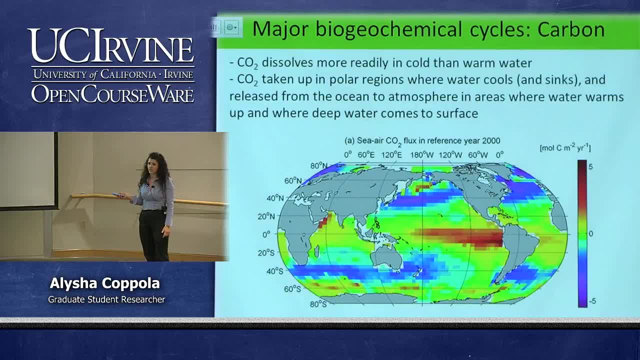 and dissolving it into the ocean, And that occurs in the colder air And you're releasing CO2 out from the ocean in warmer temperatures. So that's what you see in red. So with warmer temperatures we may not be able to sequester. 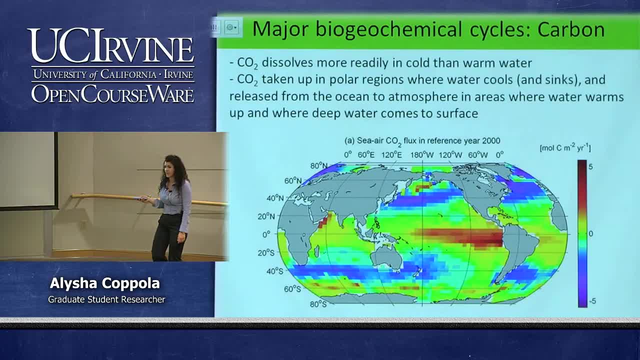 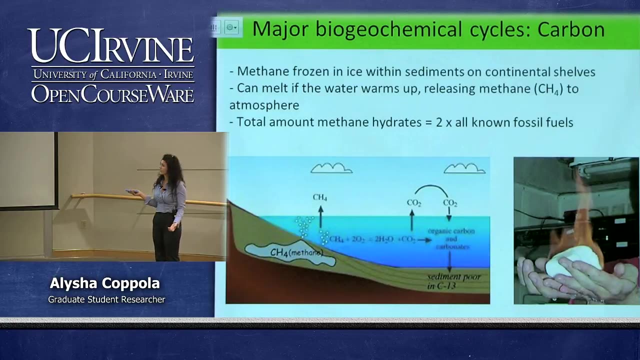 or draw in as much CO2 in the atmosphere as we have, And this is really important because this uptakes about 20% of the CO2 in the atmosphere. Another feedback that I previously mentioned is warmer ocean temperatures can thaw these methane hydrates. 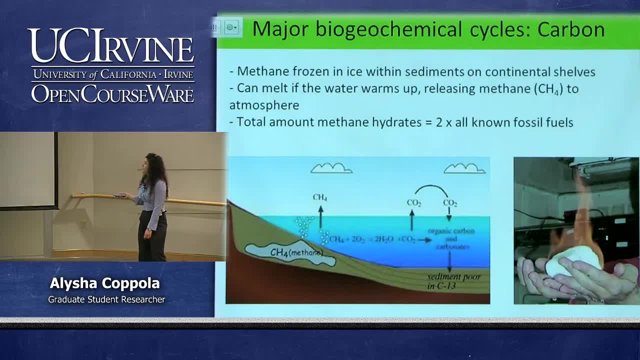 in the continental shelves and sediments. So there's about two times the amount of methane dissolved- I mean not dissolved- contained in these methane hydrates, And we're warming these temperatures. That's a huge amount of methane that we can release back. 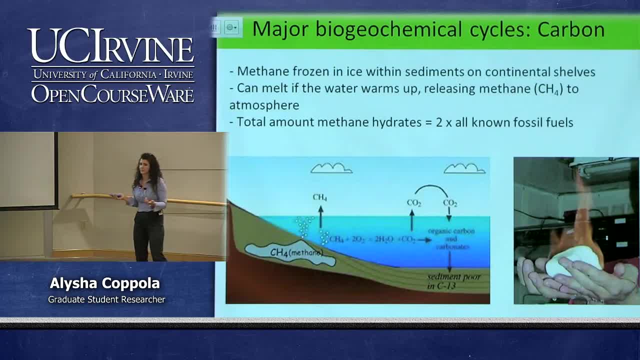 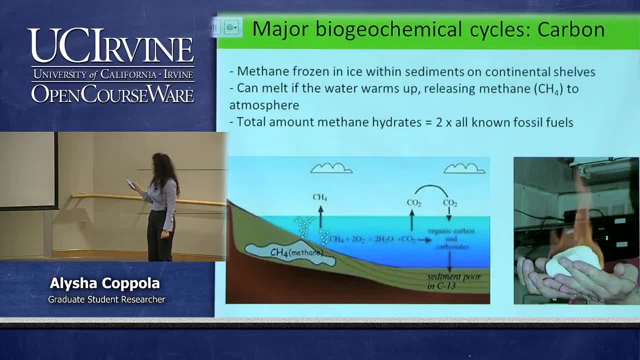 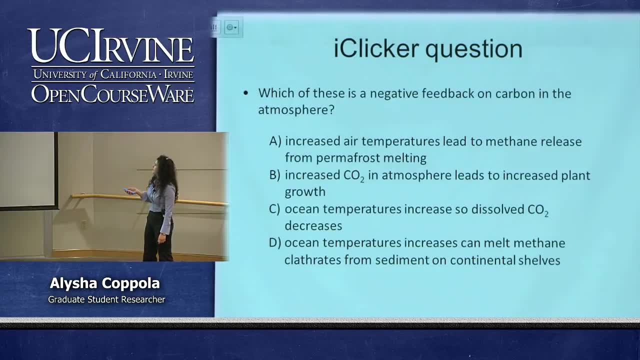 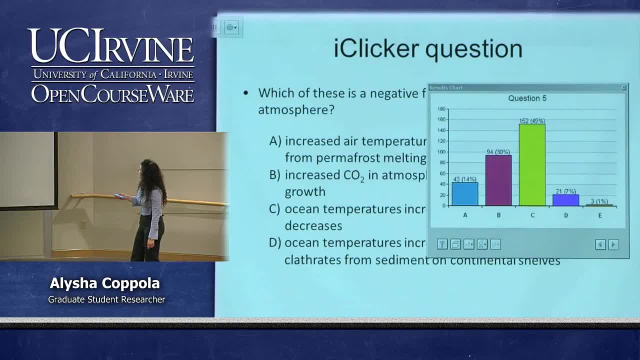 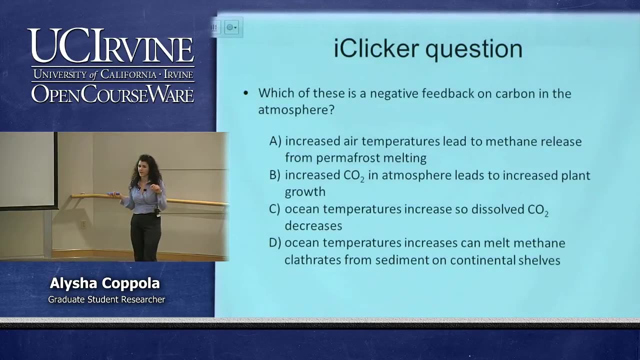 Okay, great, yeah, so C is the negative feedback. so when ocean temperatures increase, you're not able to remove as much CO2 from the atmosphere because you're not able to actually dissolve all that CO2 in the ocean. So the ocean's not able to take up as much carbon as if it were a colder climate system. 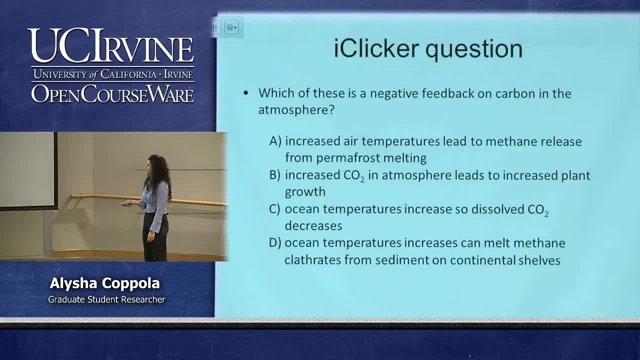 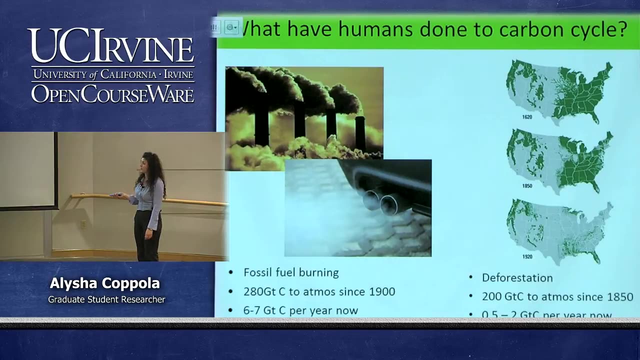 So that would be the negative feedback, because it actually yeah, okay, oops, okay. so what have humans done to the carbon cycle? So we've increased the amount of carbon in the atmosphere by adding 280 billion tons of carbon. That's 1990, and we now add 6 to 7 billion tons of carbon per year now. We've also changed the way we've used land by deforesting. So in 1620 there was more forests on the US since the 1920s, when we've started changing the way land is used with the inputs of crops and cutting out a lot of forests.